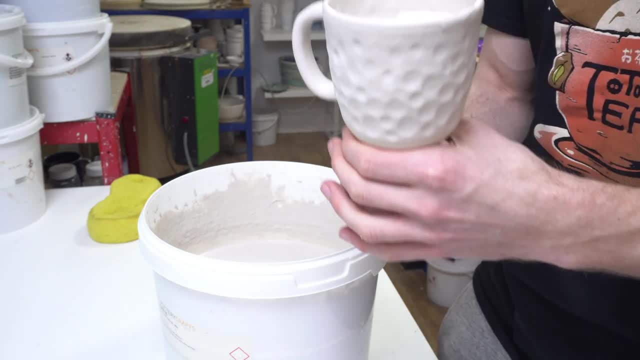 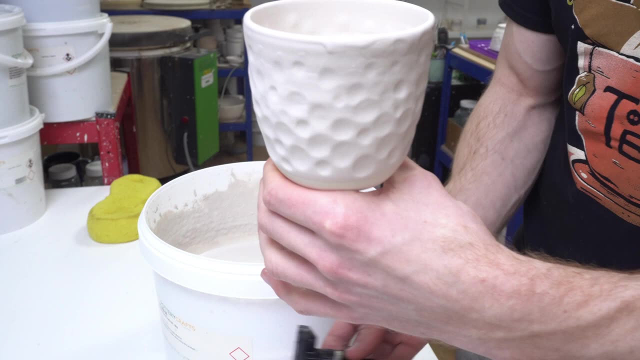 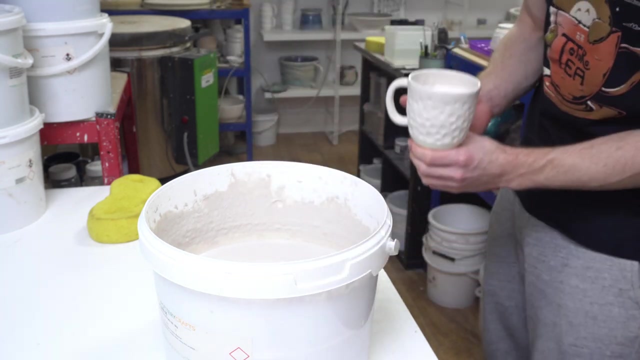 across the whole thing. so that's one thing you can do. if you get the drips, after you turn it over to get it off the dent puller, I grip around the edge, release the dent puller and then you've got your mug. you can now take from the bottom and set aside and I will let it dry up for. 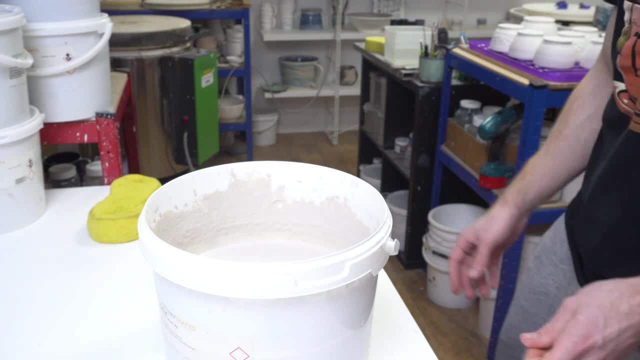 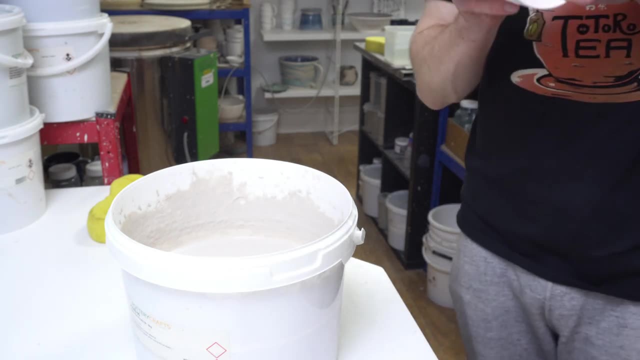 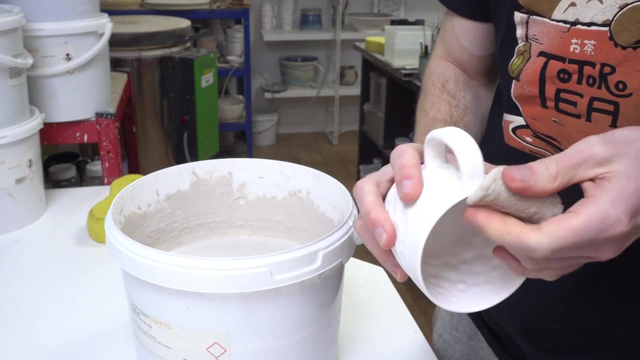 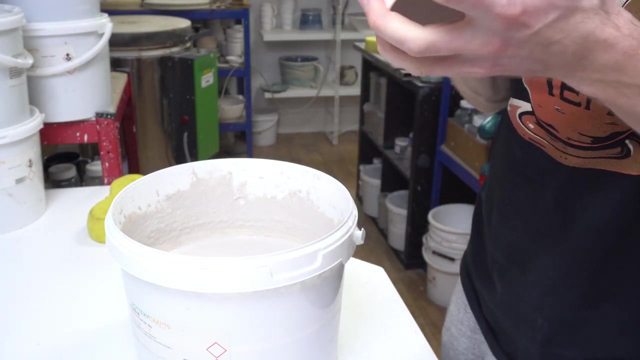 a couple of minutes while I glaze everything else before I do the inside glaze. but before I do the inside glaze I'll talk about what the kind of the main tip of this video, which is weighing your glaze. and this is something I had the idea of ages ago and I just couldn't be bothered to do. 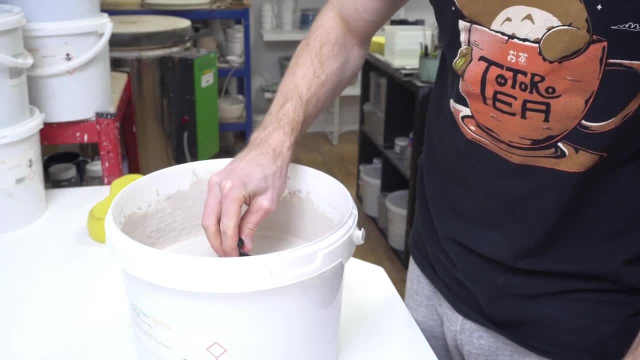 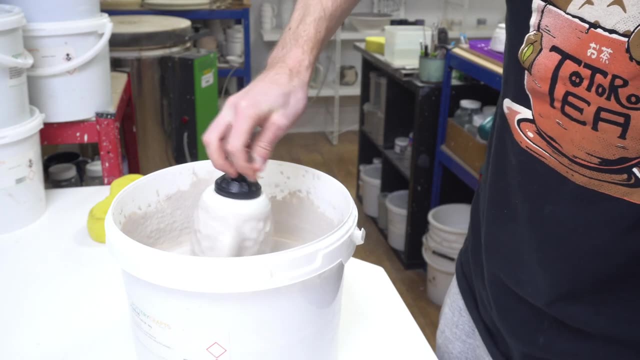 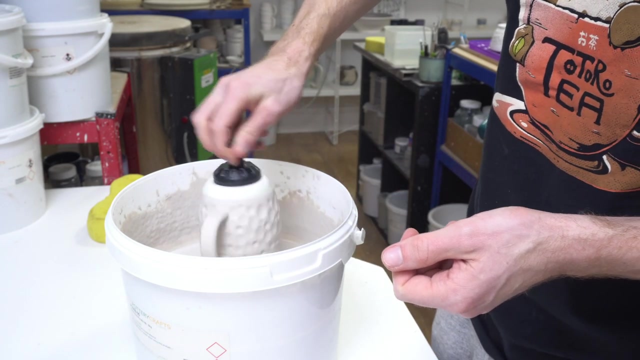 and I started doing it, which I think it was while I was doing this ceramic materials workshop class, um the advanced one, and I was working on floating blues and this is going to have a floating blue on the inside. they are a particularly sensitive glaze um to thickness. so if you want to get, 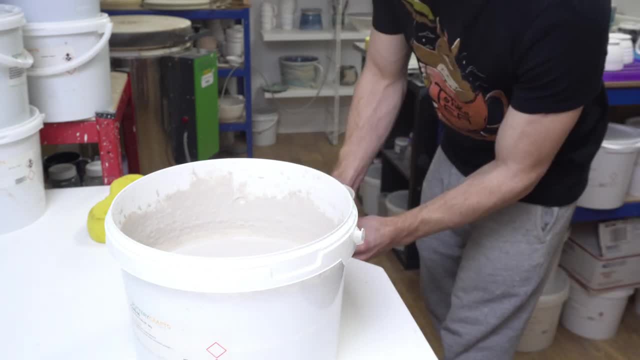 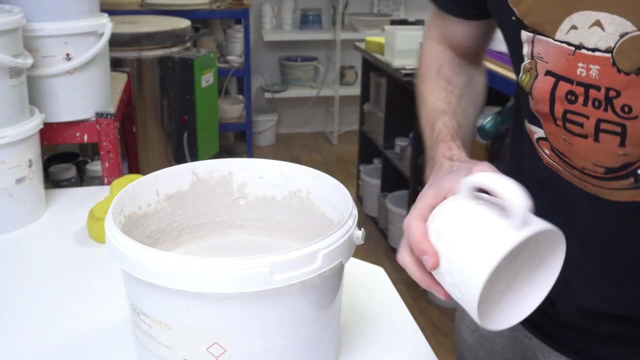 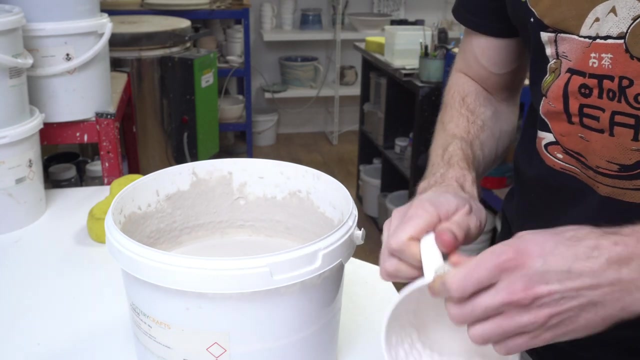 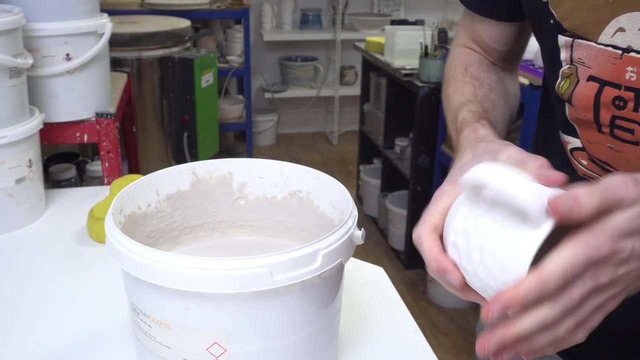 um, the color and the movement that you expect. it has to be applied at the thickness you'd expect to be applied at the thickness, and I was doing a bunch of tests, so I think I've fired something like 100- 200 test tiles and basically you can't learn anything from the test tiles unless they're consistent across applications. 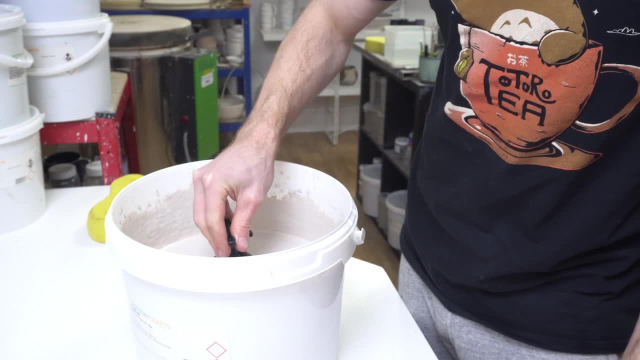 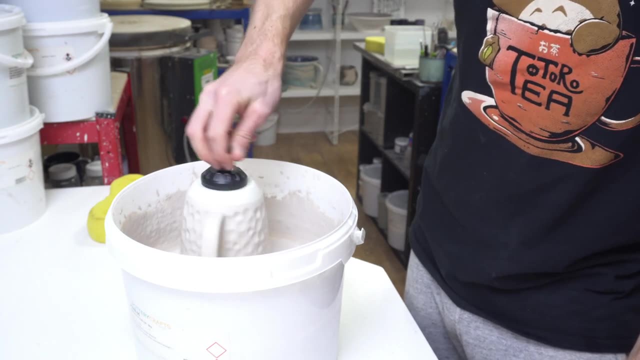 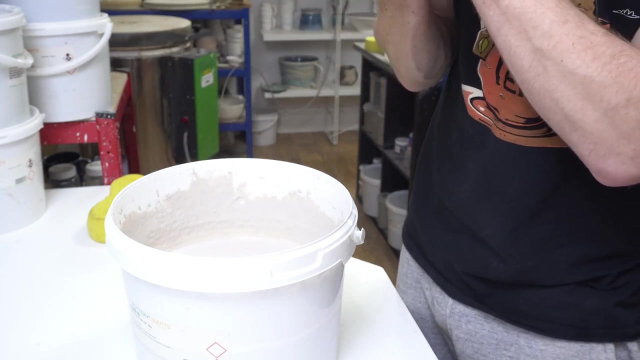 and if you're mixing up different recipes they'll behave different ways. so different blades of the ingredients kind of gel up and get thicker in the bucket at the same specific gravity. If you're not familiar with the term specific gravity, it basically just means density relative to water. but with something like this, where 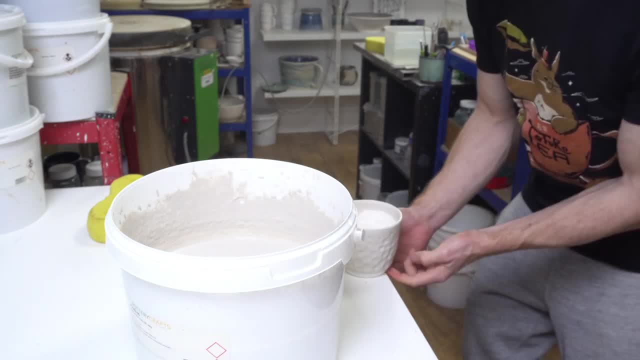 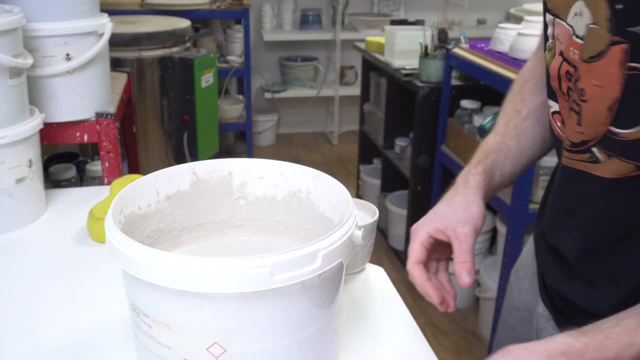 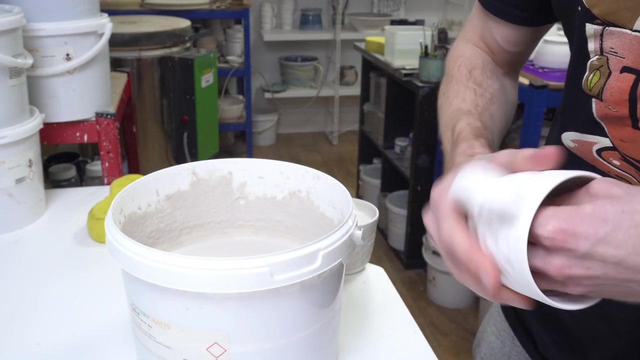 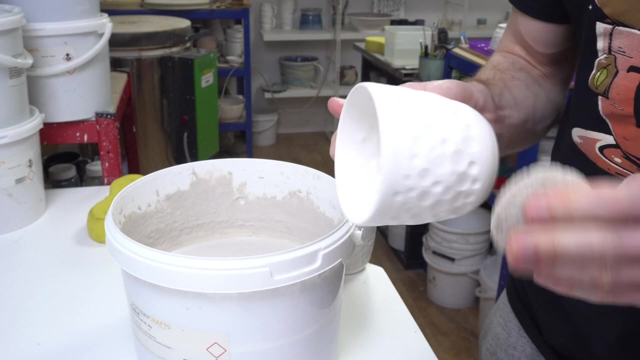 you're diluting it with water. the specific gravity is basically how well packed all the glaze ingredients are and how much water you've added to it. So obviously, glaze ingredients are rocks, essentially ground to dust. they are denser than water, so generally you're aiming for a specific gravity of 1.5-ish. 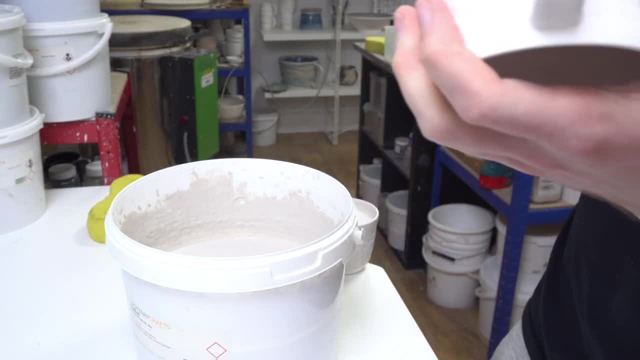 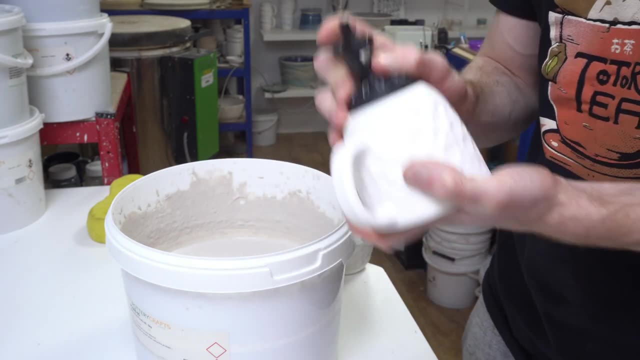 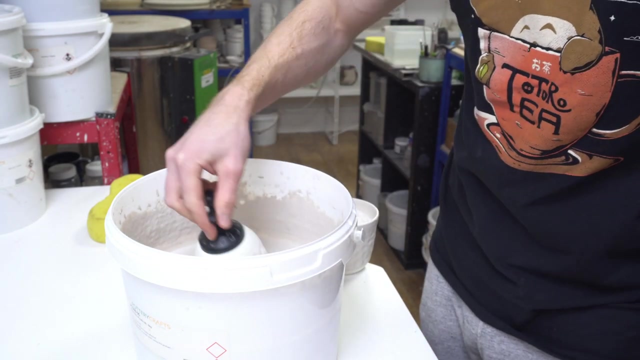 for glazes: 1.4, 1.5. What that means is it's 1.4 times the density of water. so you know that there's more things added to the water. The more water you add, the closer to one the specific gravity gets Very easy to calculate. specific 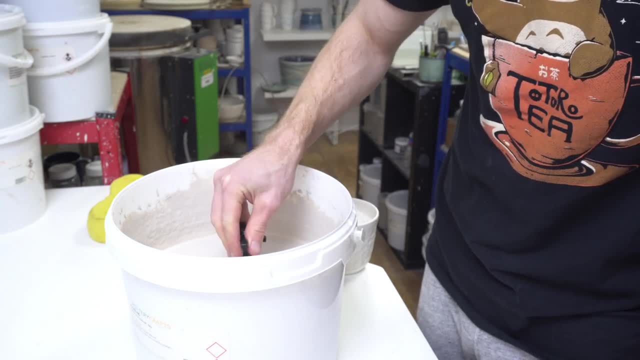 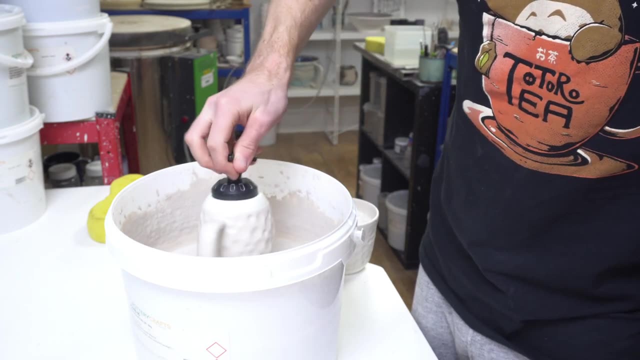 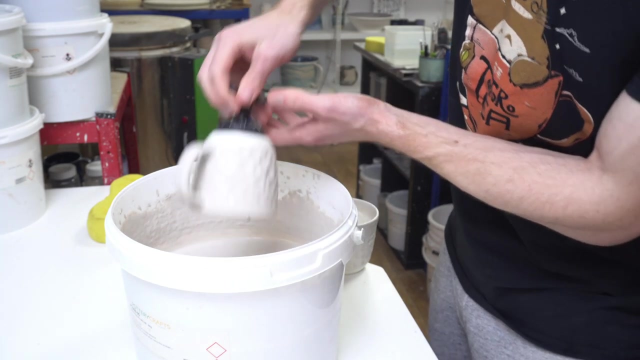 gravity. you just take a volume easiest, if you do 100 ml and weigh it. And if it weighs 100 grams it's got specific gravity of 1, if it weighs 150 grams it's got a specific gravity of 1.5.. But the point is that different. 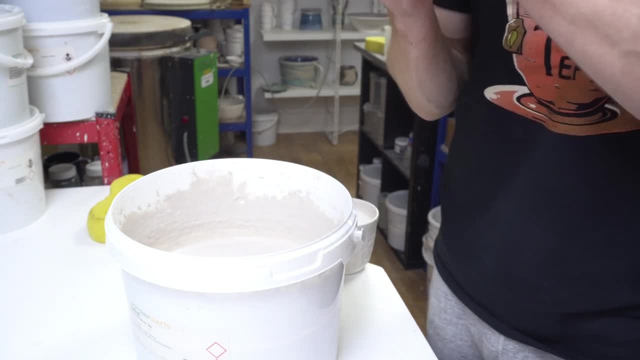 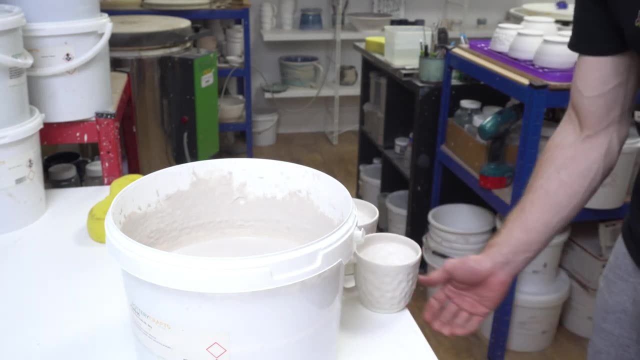 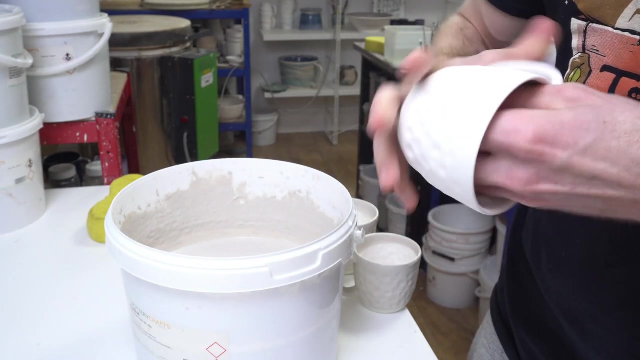 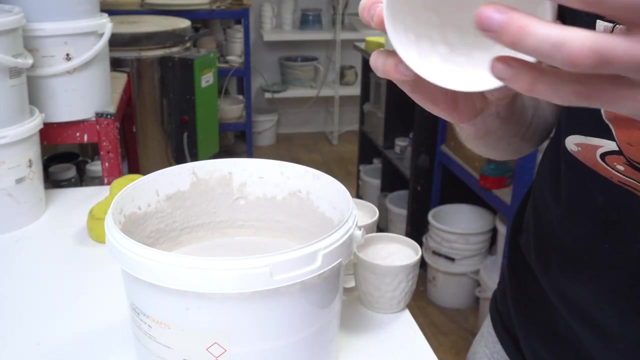 glazes behave differently. So in order to get a consistent comparison across all of them, you want to know how much glaze you're putting on your tile, And the hands-down quickest, easiest way to do it is just zero a set of scales on whatever you're applying the glaze to and apply the 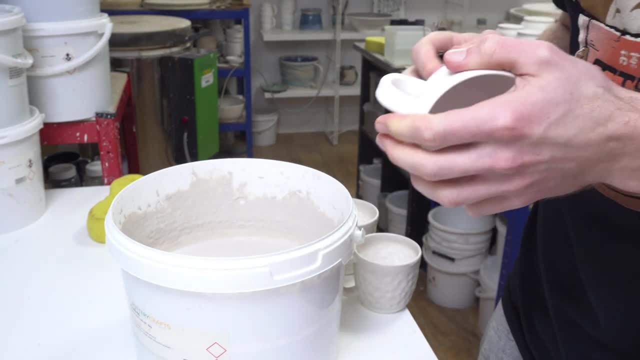 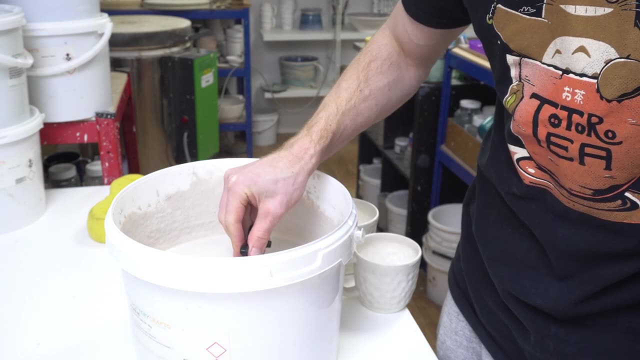 glaze and then see how much is on the test tile. And once I've started doing that for those it really became a bit of a no-brainer to do it for particularly the pieces like this where there's a bit of a gap between the glaze and the 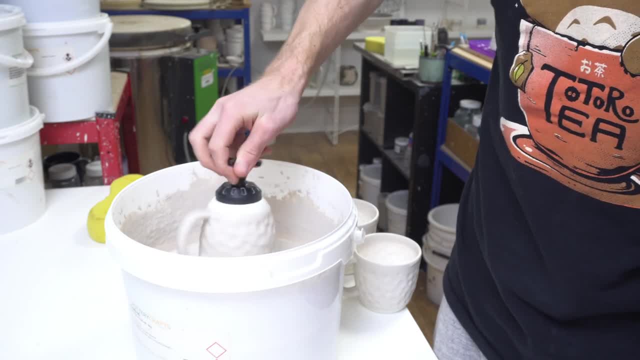 glaze. So I've just taken a little bit of a gauge and I've added a little bit of glaze to it. I've just added a bit of a scale and then I'm just going to go ahead and check whether there's any water in the glaze. And it's quite easy to do that. 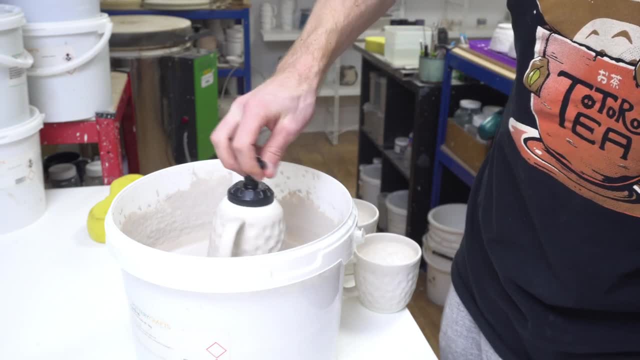 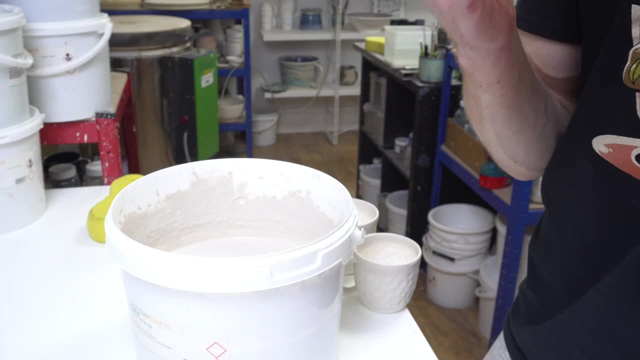 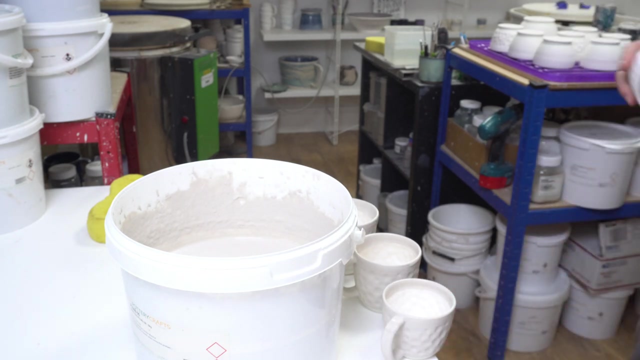 because it's a bit more sensitive to application. But it means you can check consistency across time as well with other glazes and other applications. So I will, every now and then I will just weigh a piece, as I apply the glaze to it, of one of my other glazes which isn't quite so fussy about it, And it means: 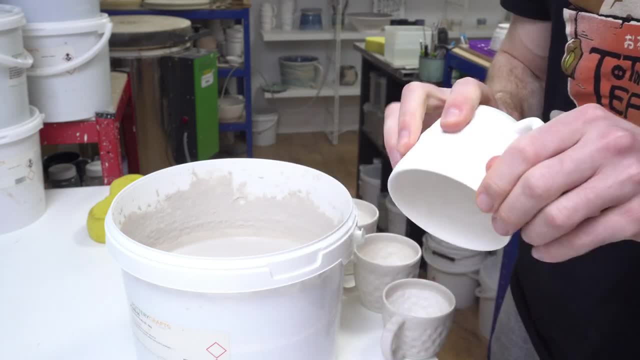 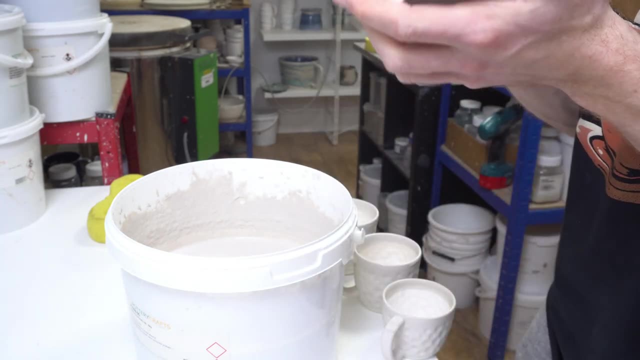 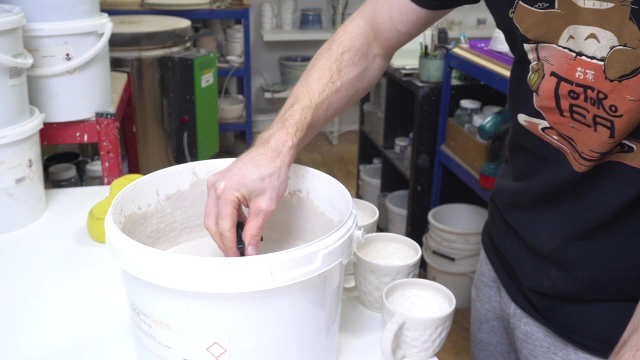 that you can check. You can do a control piece where you weigh your application to see what your application looks like, Write down the number and then just check. you know, six months time, If you're hitting those numbers with a glaze, that's diluted by the same amount, which is part of the relevant thing. 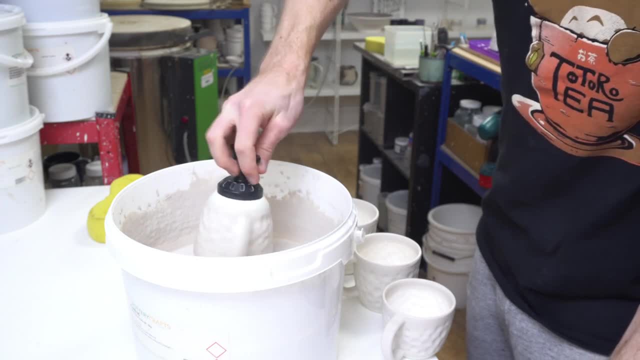 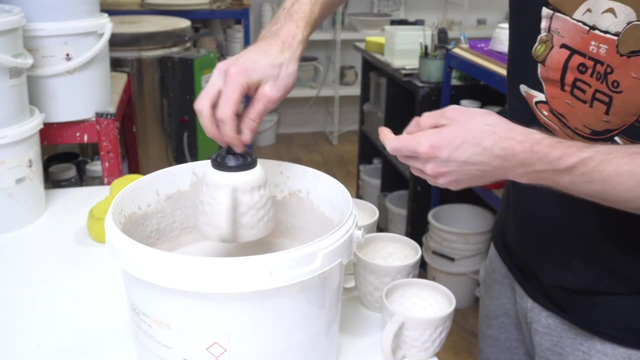 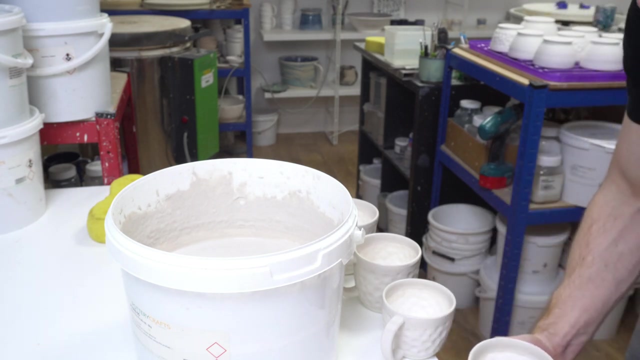 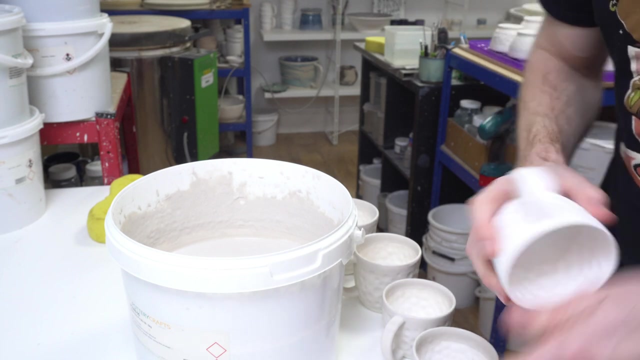 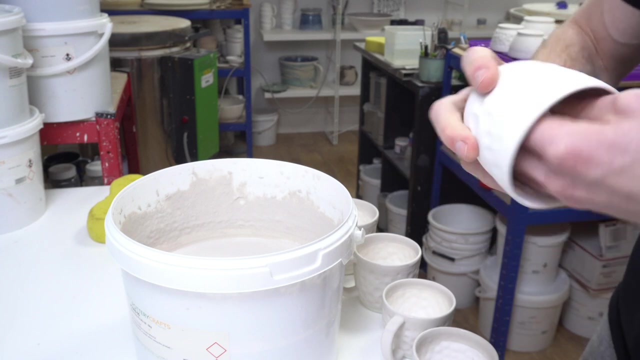 But when you know your variables for your glazes you can very easily have consistency over applications and over time. Interestingly, with the capacity measurements you'll find that they don't scale with the amount you need, doesn't scale linearly with capacity. 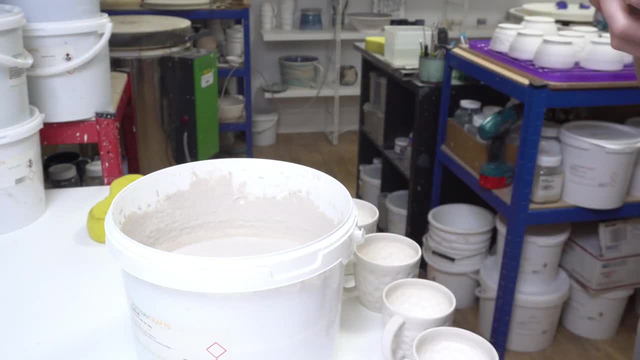 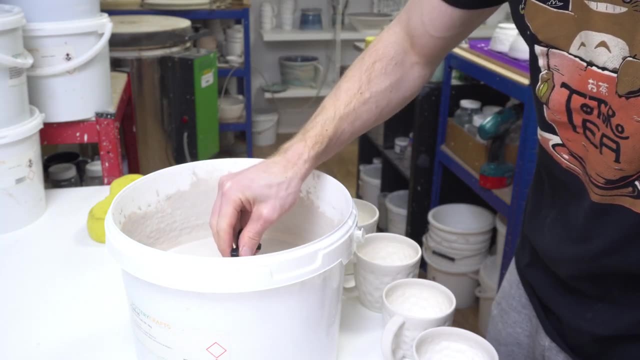 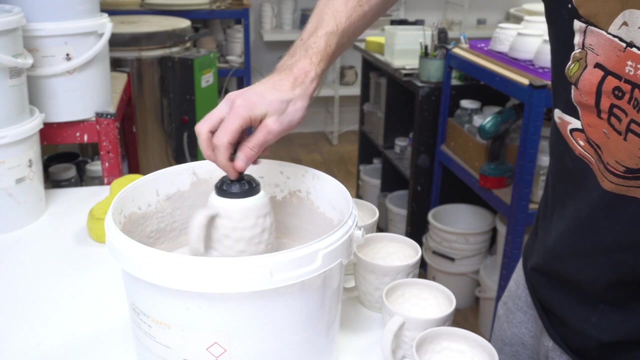 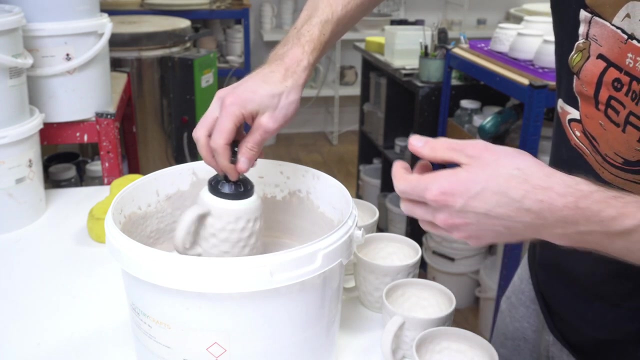 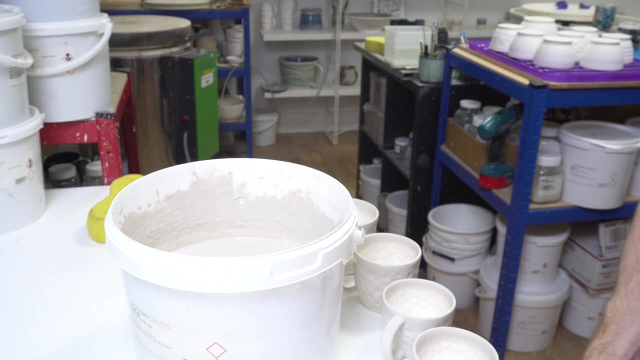 So as in my small mugs are roughly Half the size of my giant mugs. And Well, in fact there is less than half the size of the giant mugs, but the they need A little over half the amount of the glaze inside, and you'll find that gets even more pronounced as things get significantly bigger. it doesn't scale linearly. And the reason for that Is what's known as the cube square law, but it's the idea that volume increases relative to surface area, differently as you scale things up, Depending on the specific shape. but they don't scale together, which is why- small animal- you can't, you couldn't just scale a small animal up to a big animal, because things wouldn't work the same way for it. 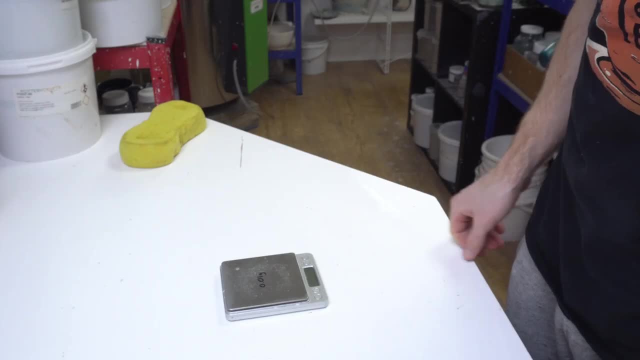 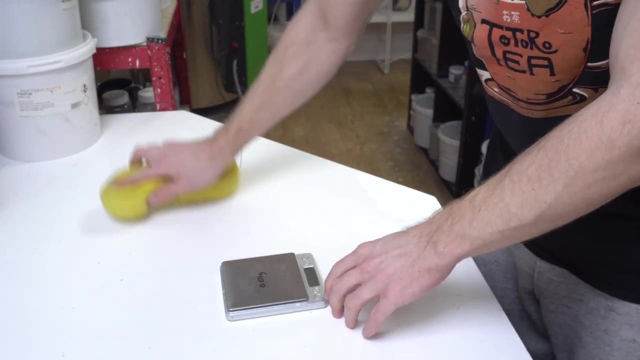 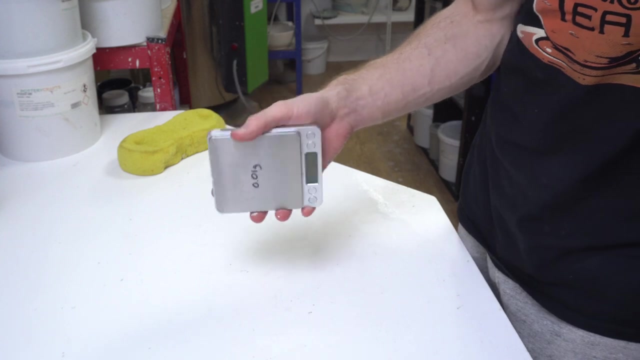 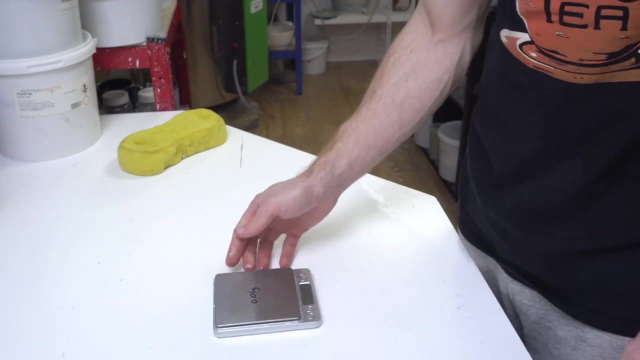 That's why same applies to these, Right, so this is how I do the inner place. This is the relevant part, really, and- and I'm just using one of these really cheap 500 grams by 0.01 gram scales, But there's, these generally come in two formats. 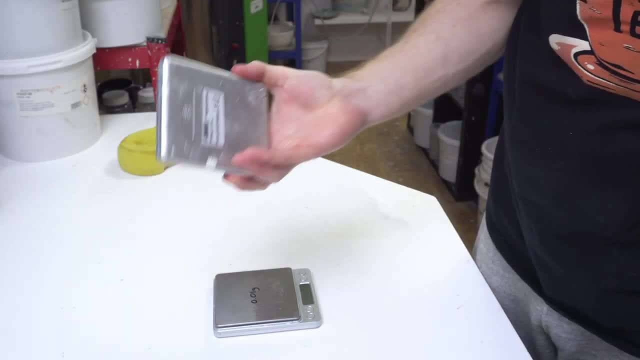 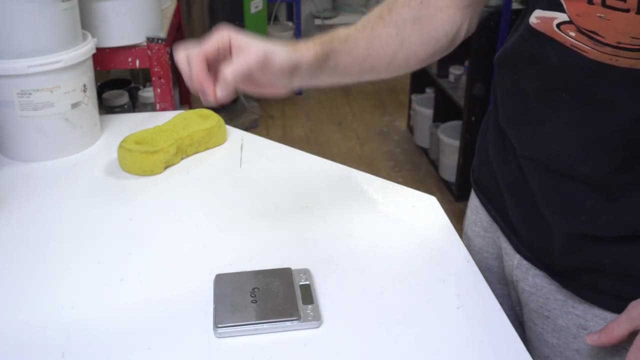 That's a 0.01 gram ones and the 0.1 gram ones, and they go up to three kilos. So I like having The two of them. This one's more precise but with a lower limit, Obviously that one goes a bit higher and then 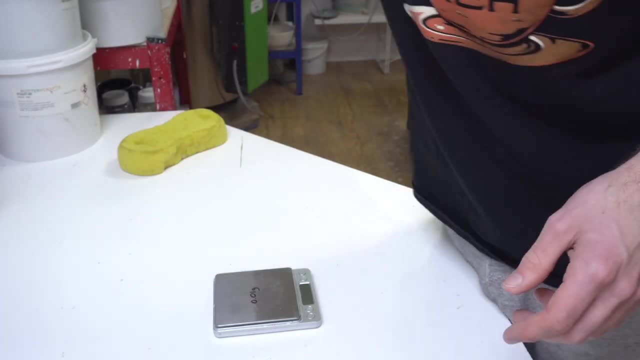 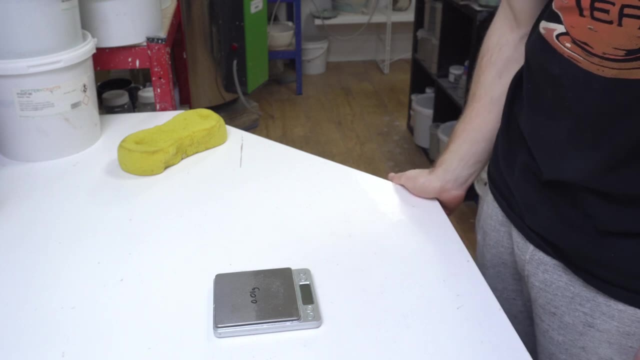 The scale is a 10 kilo kitchen scale, So for each one you lose precision as you gain weight, and they're all about £10.. It's nice having one of each of them. They work really well. They're accurate enough. 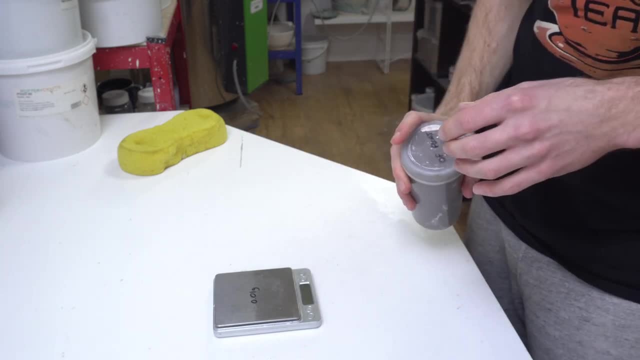 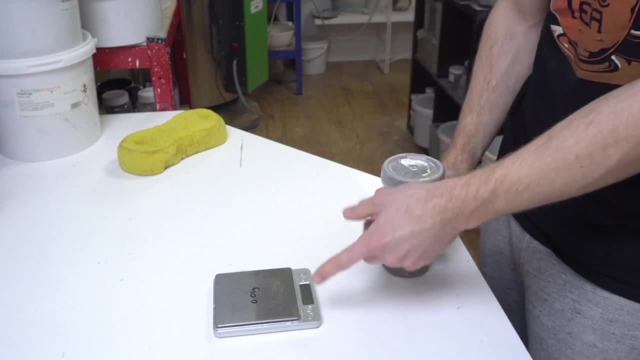 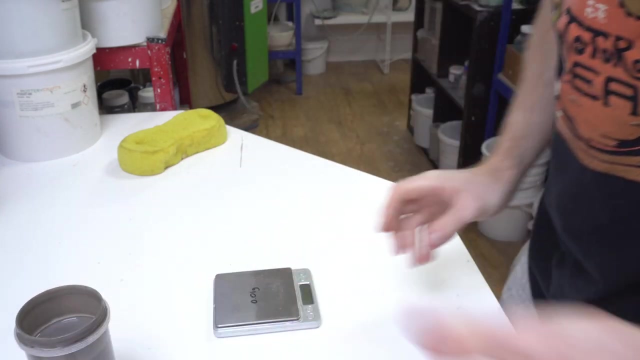 They're not going to be as accurate as an expensive scale, but you can spend hundreds Or thousands of pounds on the scale If you want real precision. that one's good enough for pretty much everything, Certainly good enough for this. So that's what I'm using. 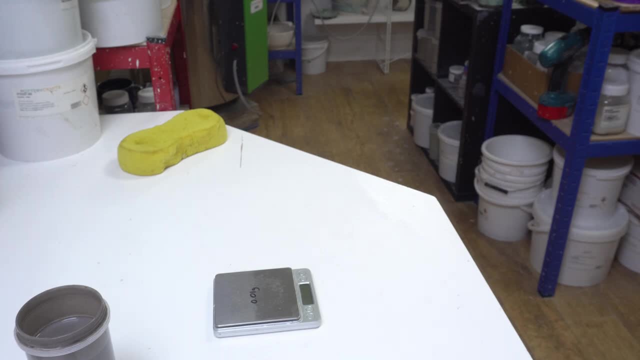 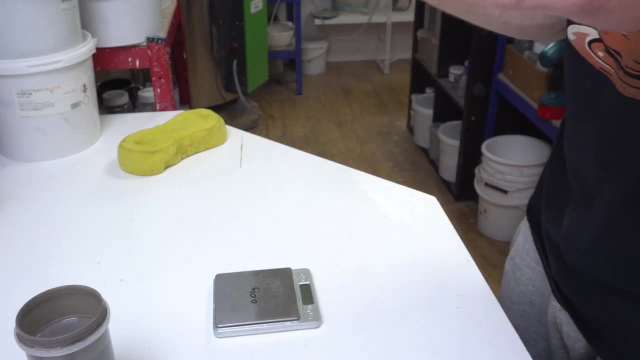 I will glaze a couple of different sizes So you get an idea of how much glaze I'm using for each size. This is with a floating blue, so that I'm doing quite a thick application of these And you do need to know how much water you've added. 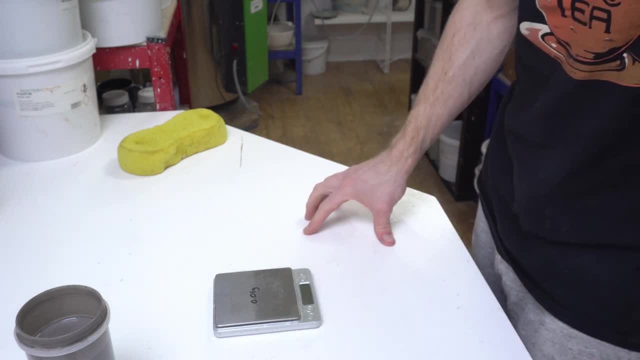 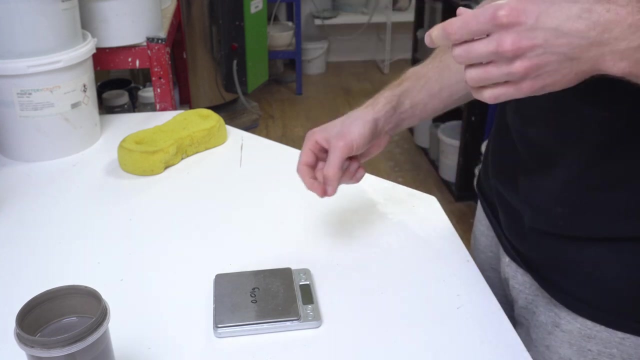 At least approximately. So I start diluting my floating blues one to one, glaze to water. So for a kilo of glaze mix I will put a kilo of water in, And then generally that is a bit on the thick side. 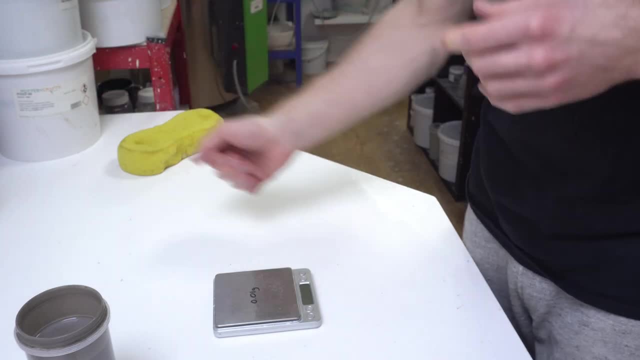 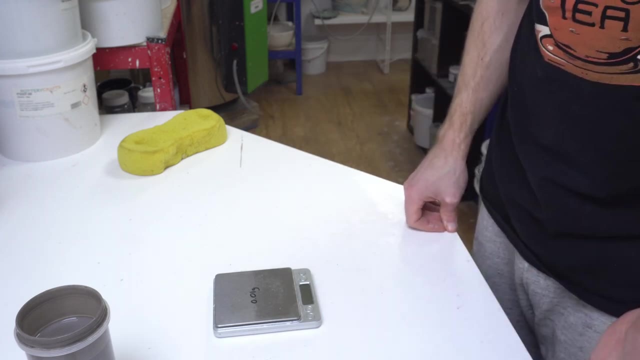 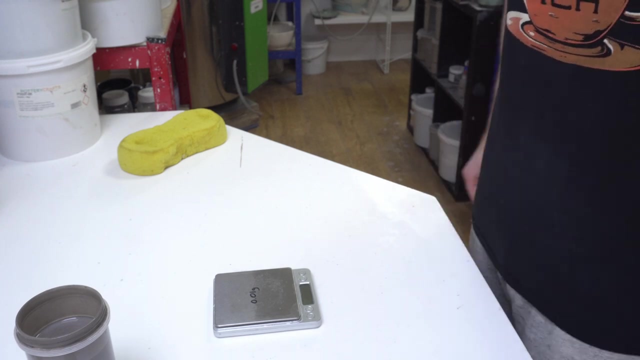 So I will add a little bit more water as they thicken up, But that's a nice starting point. You can measure specific gravity, as mentioned in the previous, A little bit, Which will again give you consistency, but it's not the only thing that matters. 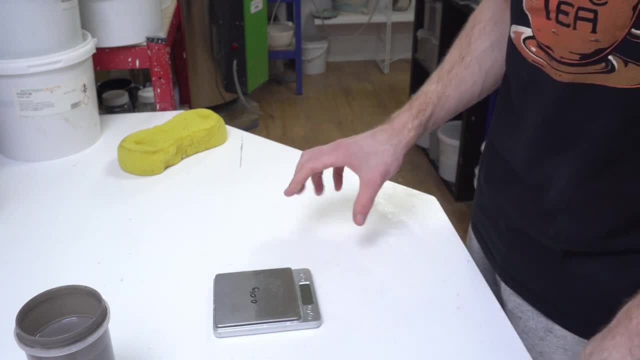 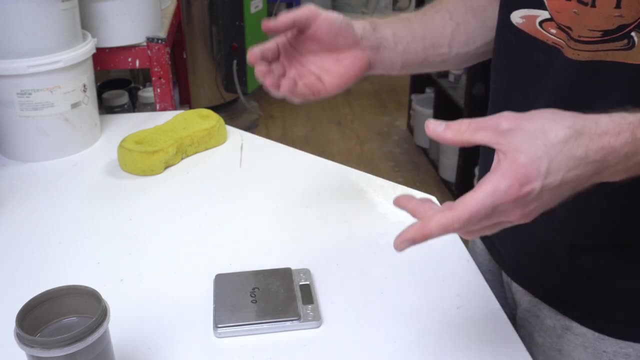 A lot of people get very hung up on specific gravity. It's a useful measure, but it's not the most important measure You want to know. it's a trade-off between how the glaze is behaving, So how essentially, how thick it is, how viscous. 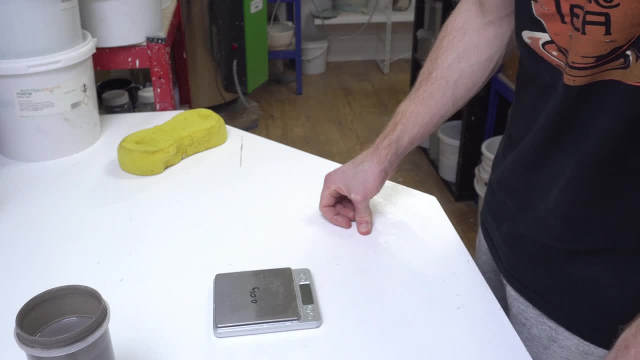 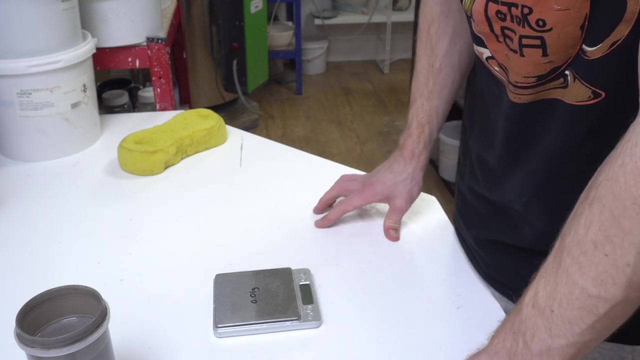 Because it's no good having the right specific gravity if it's not applying properly. And then how much your bisque wear is taking up, Which will be dependent on your clay and your bisque temperature. So don't worry too much about specific gravity, but it is a useful measure. 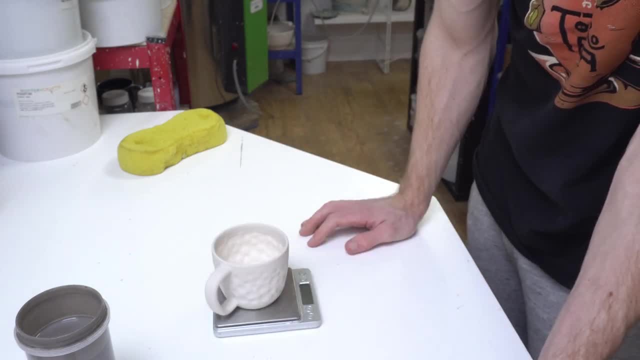 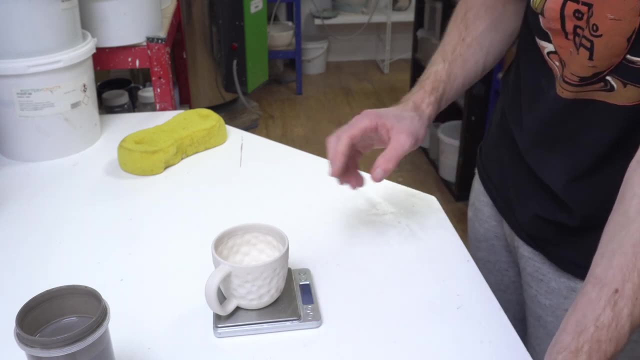 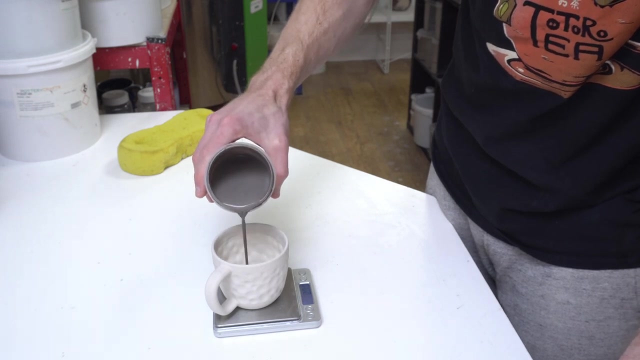 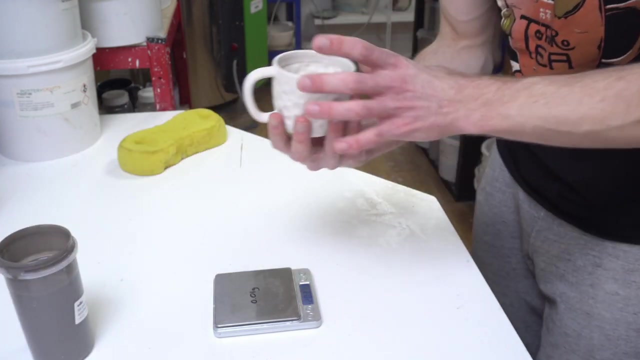 This is a small mug. Fired capacity will be 250 ml thrown with 250 grams of clay. I will put just under 20 grams of glaze into that And that's 20 grams total weight, So including the water. The nice thing is it doesn't matter if you're a gram or two out. 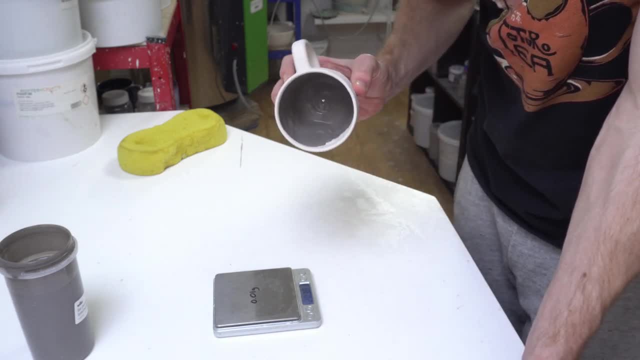 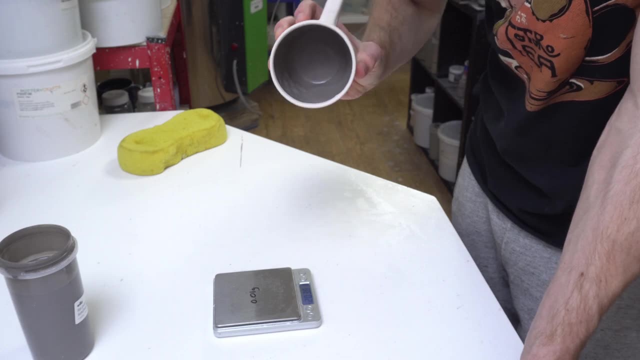 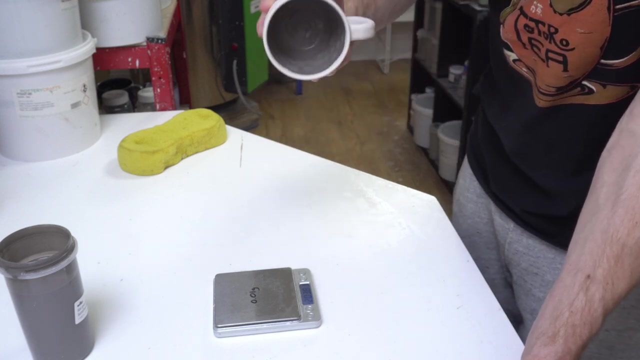 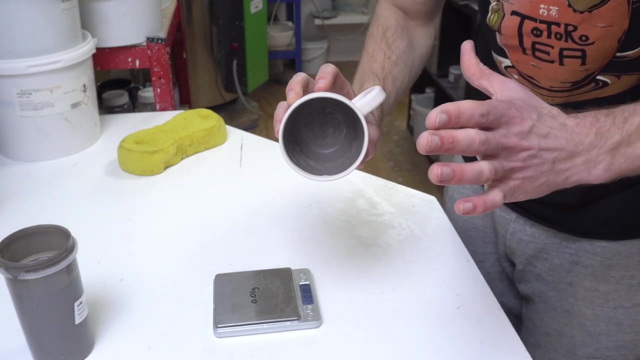 What you're really looking for is to not be wildly out with these. Obviously, that is in part because this glaze is inherently quite variable. My application doesn't need to be perfectly even. What I like to get is evenness around the piece rather than constant across the whole thing. 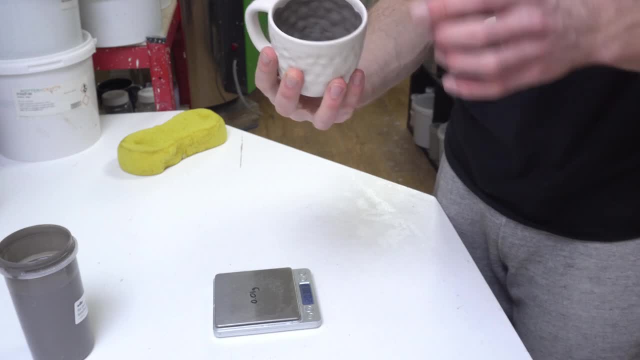 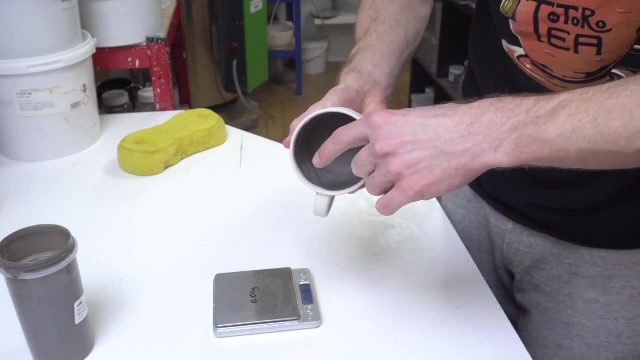 Because the idea is that I want it to flow down. So what you saw me do there was pour in. I swirl round to get the bottom covered. I twist round to get up to the rim Once I've gone round and back, I then swirl to cover the bottom again. 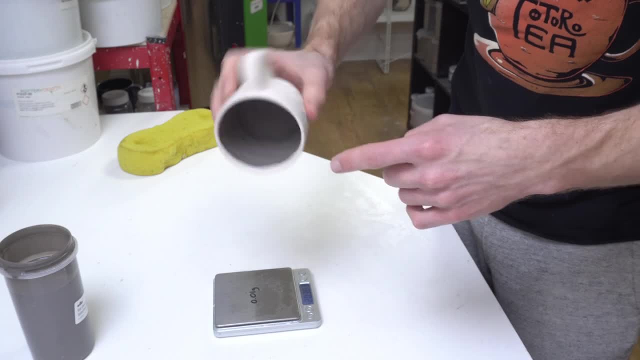 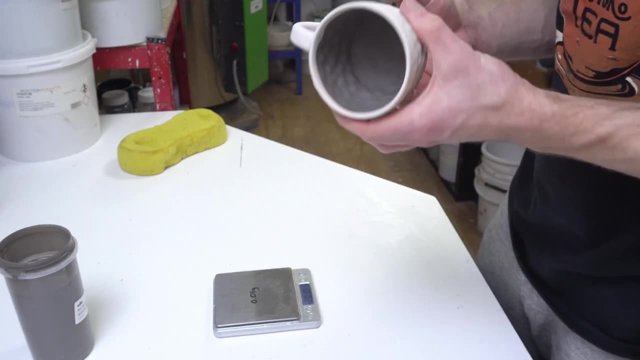 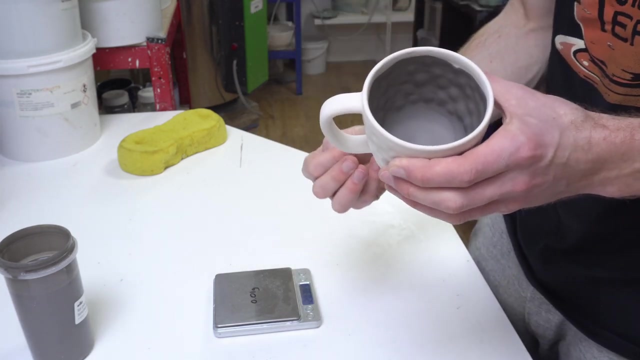 And then any remaining glaze. I just turn it like that to run it round And round in bands until it firms up, And the reason for that is: you don't want too much at the bottom, Because that's where it's going to naturally want to pull. 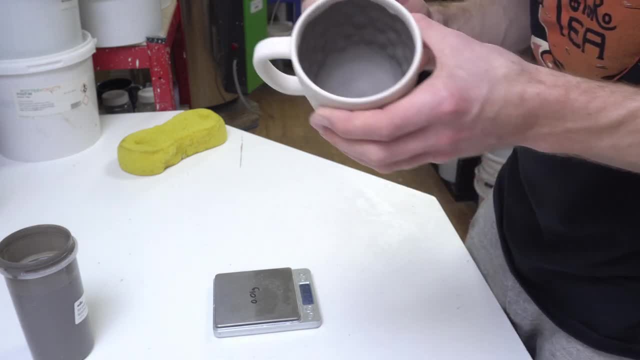 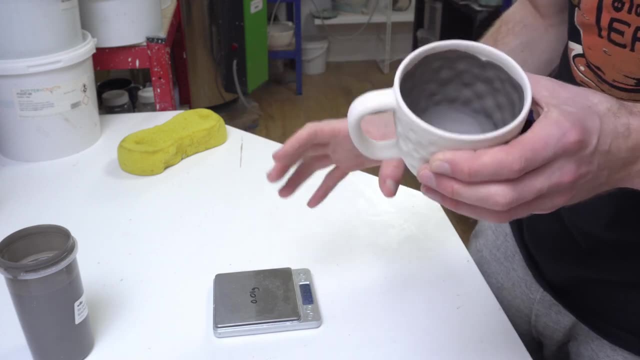 And if it's too thick it will start to craze, And that's pretty much across the board. Even if you've got a glaze that doesn't craze much, that fits your clay well, If it goes on too thick it will lean that way. 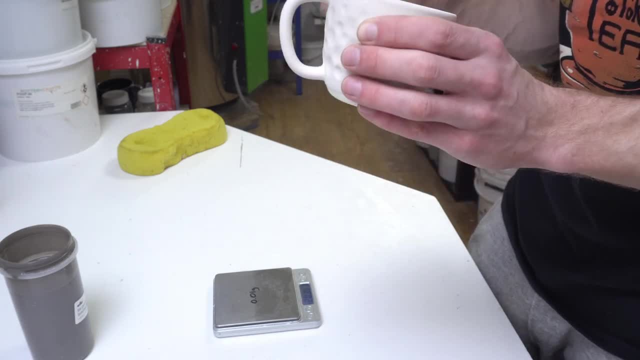 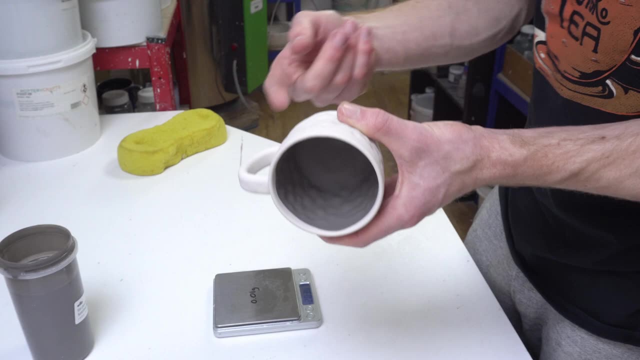 Especially in something like a mug, where it's going to have boiling water poured into it. So you want to avoid too thick an application at the bottom, And that's very easily done. So what you do is you try and keep it on the walls of the piece where you'll get that movement over the pattern. 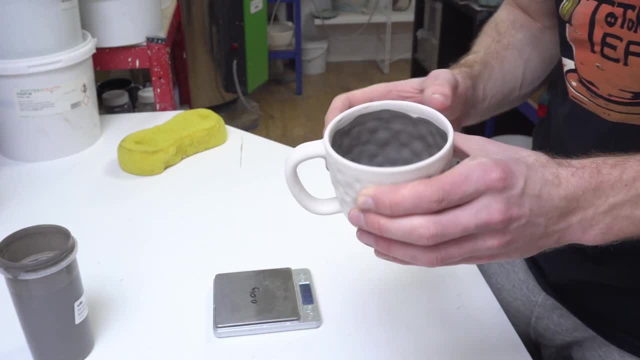 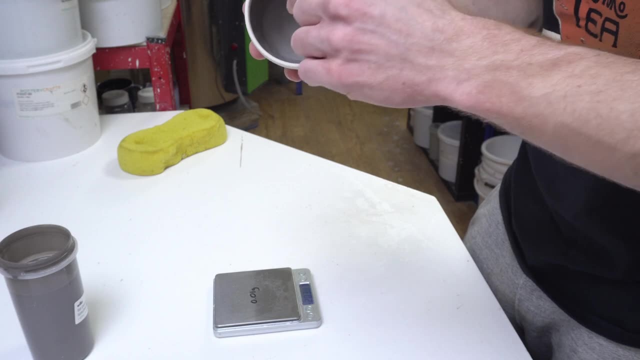 That's what makes it a pebble in this case. But the pebble, peacock eye, nautilus, impulse- they all rely on the fact the glaze is flowing down the piece. So you want most of the glaze up around the rim. 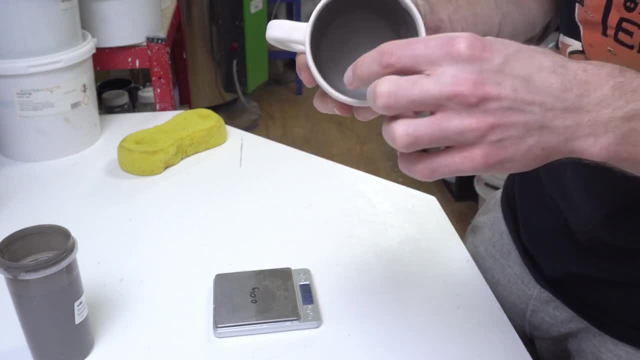 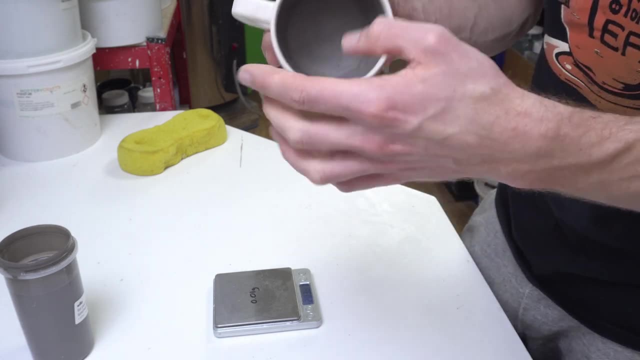 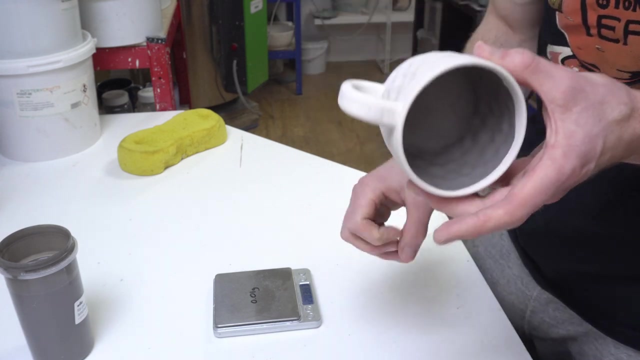 You don't. from my experience I would say with my application you don't want too much in the overlap. You're better off having most of the floating blue just below the overlap, because there's already the other glaze there And once you get into too thick an application you're at risk of crawling. 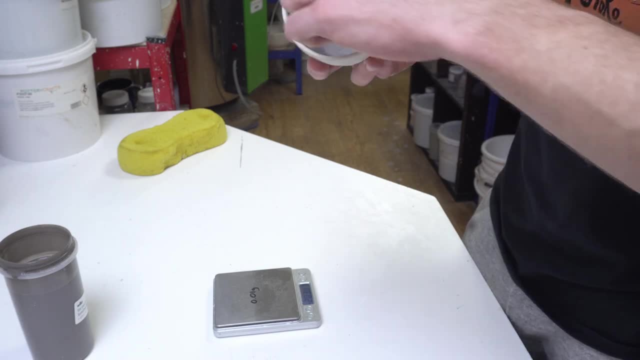 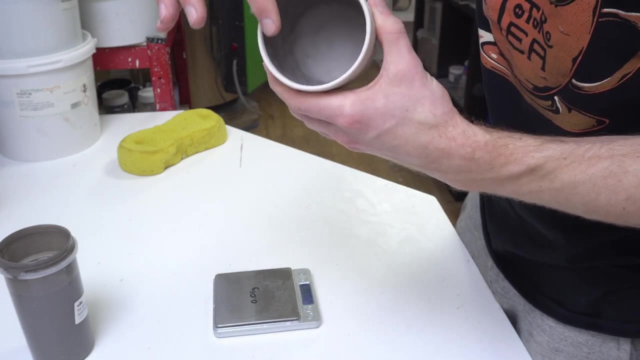 which can be resolved by chipping off. When it starts to peel, you chip it off and reapply it, But it's best avoided. So try not to get too much on the overlap. just overlap slightly and then dump the rest of the glaze around. 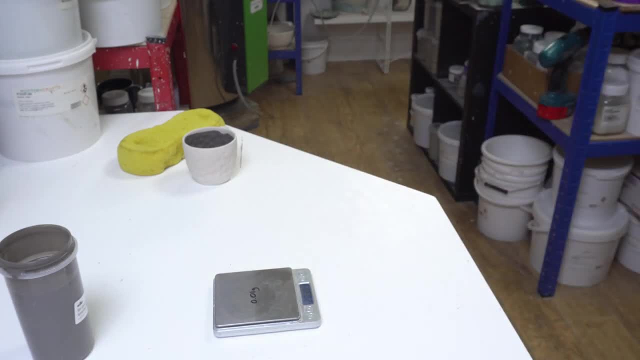 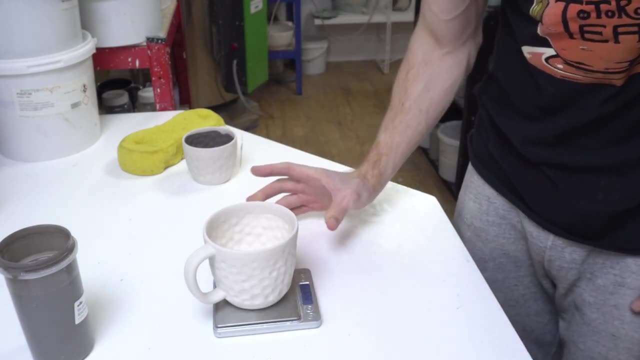 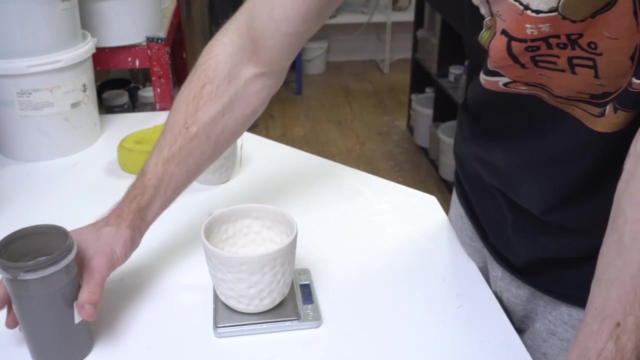 So that is on a small piece, And then we have actually I don't know what size this is, I think probably just a large, yeah, So large I'm going with 450 grams, capacity of 450 mil, So nearly double that. 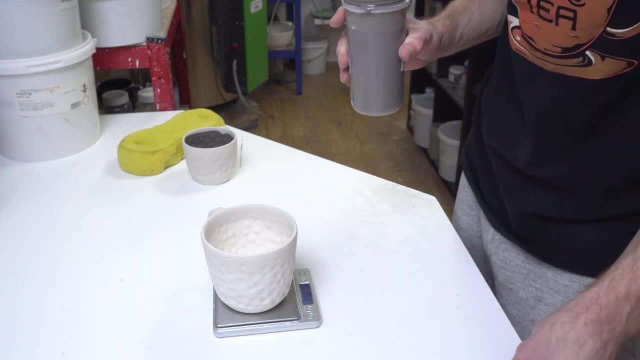 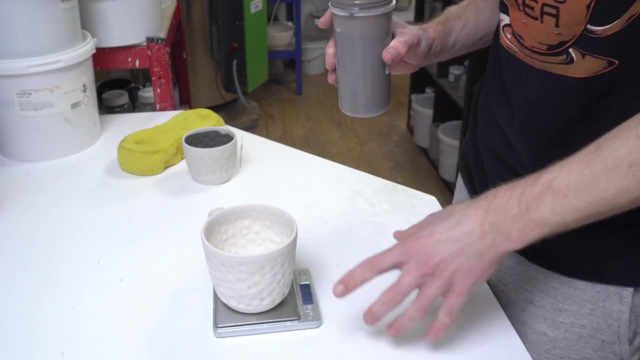 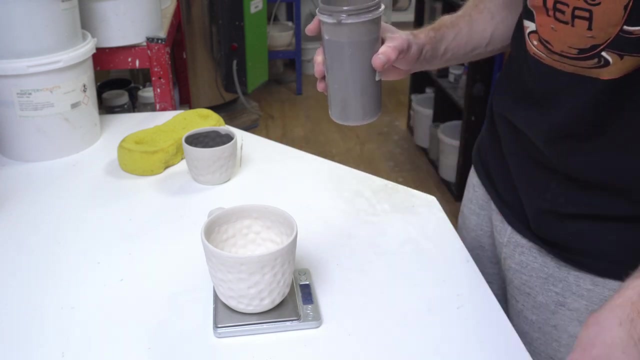 But I'm going to put generally low 30. So I'm about 33.. No, not even that much. 30 grams for these. So 30 grams and basically you're looking at nearly twice the capacity. half again as much glaze, just because of the way it works. 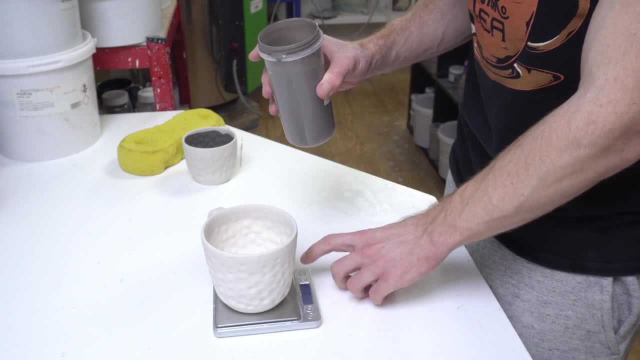 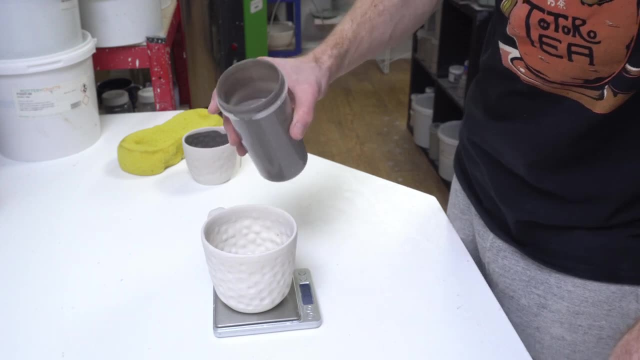 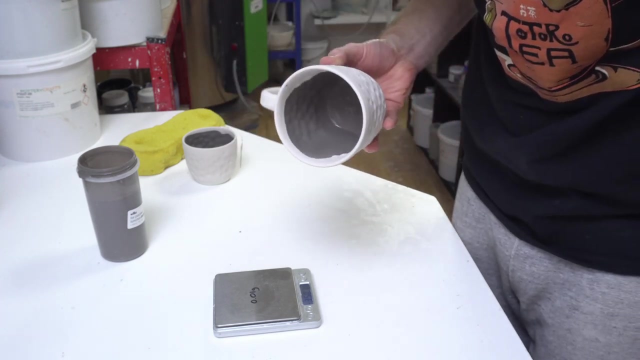 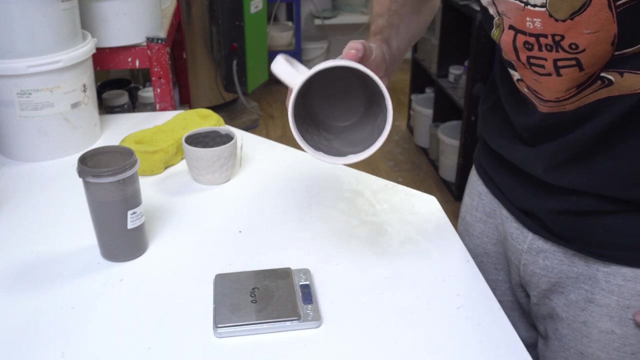 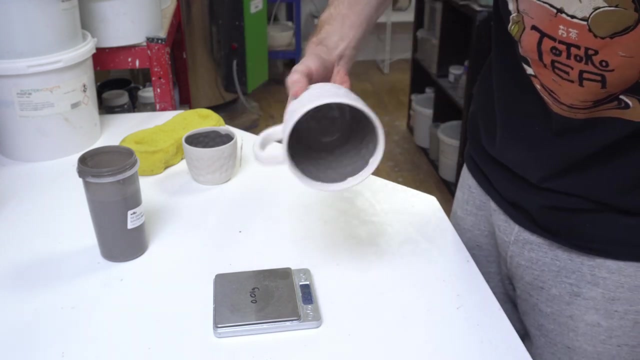 So zero the scales, 30 grams and a little bit of measure. Swirl it around, Roll it around at the top And back again, And then even coating on the bottom, and anything that's left gets redistributed up the walls. 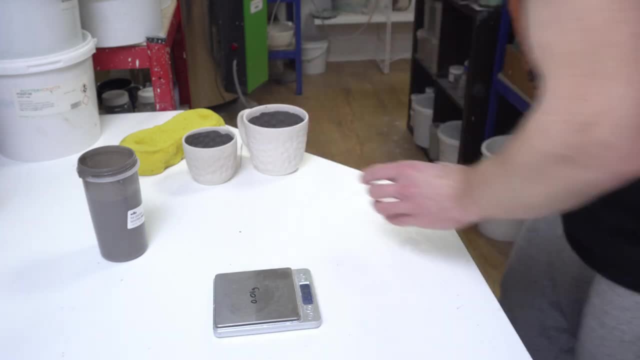 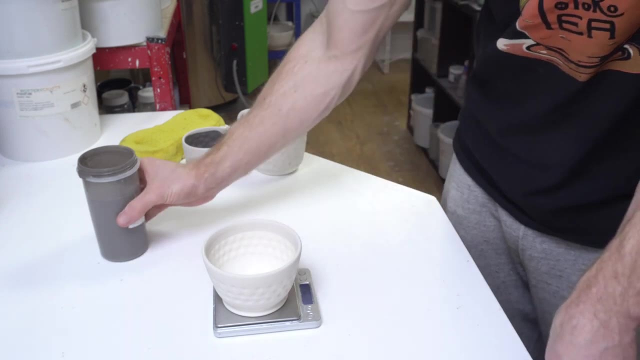 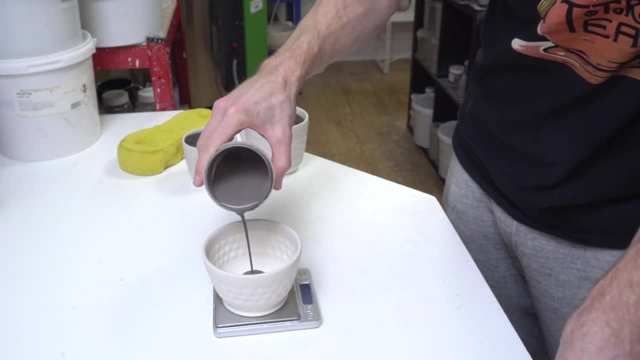 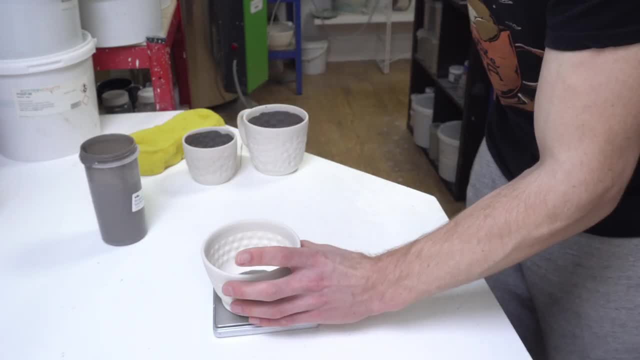 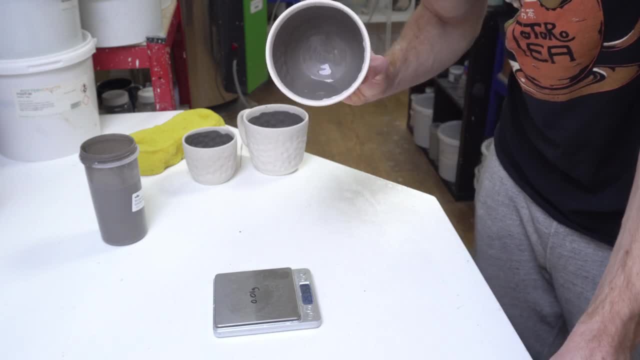 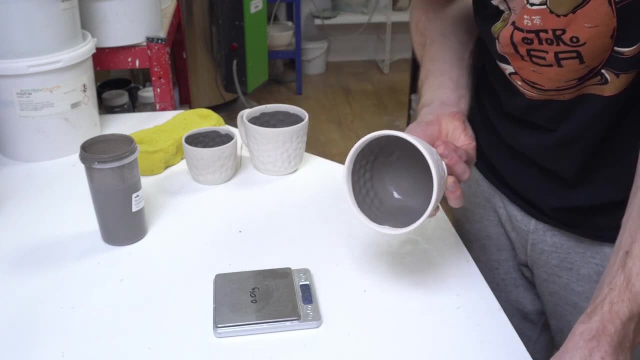 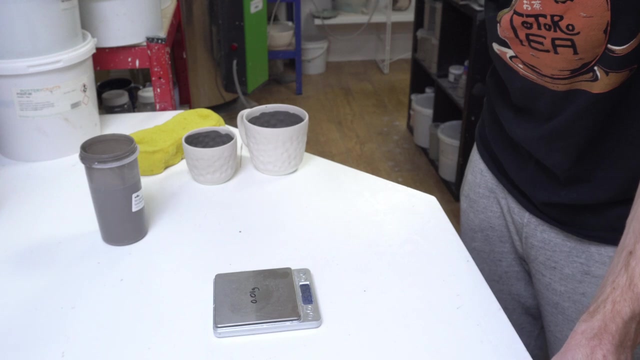 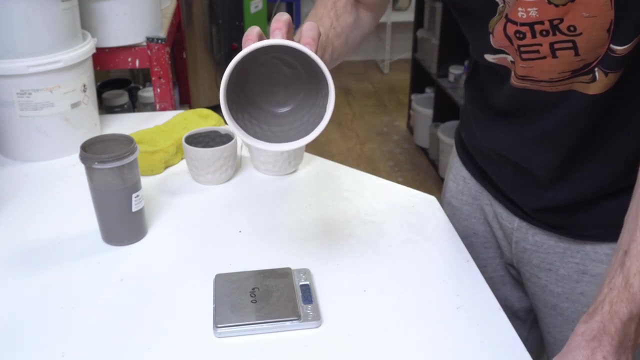 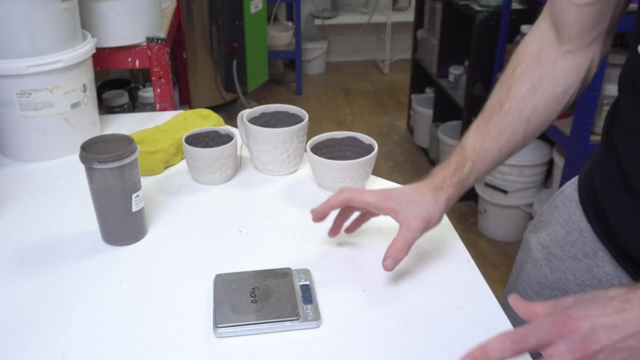 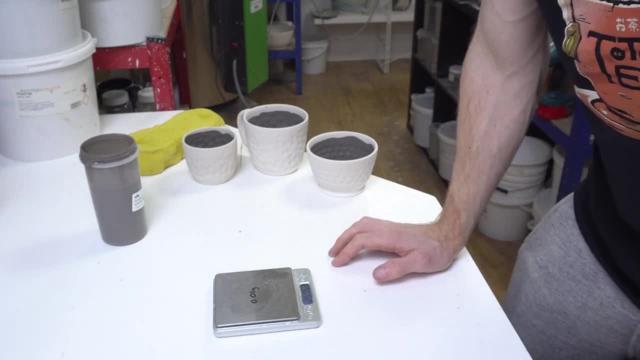 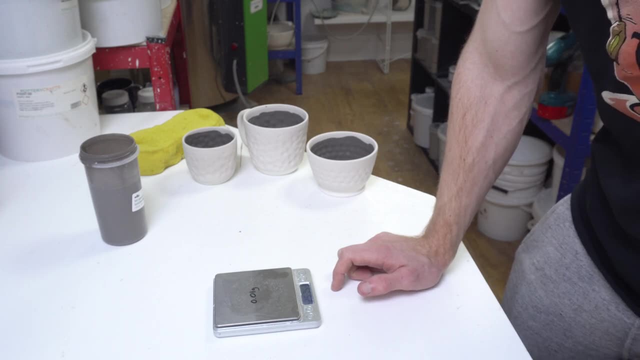 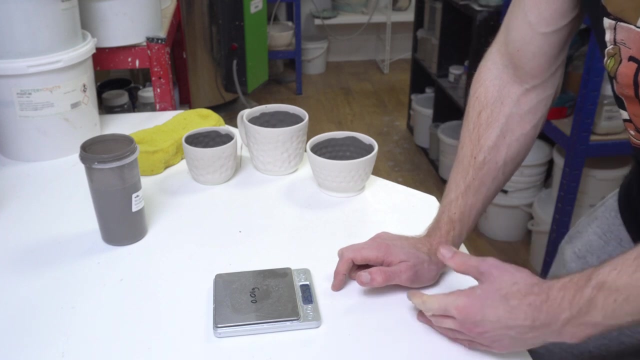 or you want to have consistency over time. you don't have to do this with every single application, but I tend to for mugs, because they're enough effort and you don't really want to either direction too much or too little. it's not great. so the amount of time you've put into the 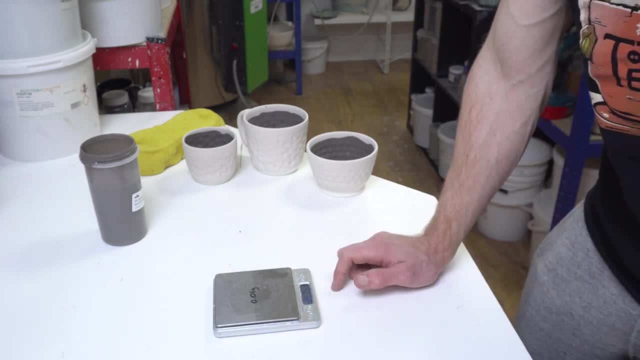 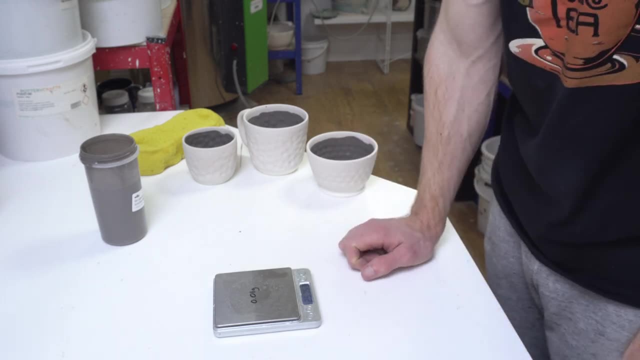 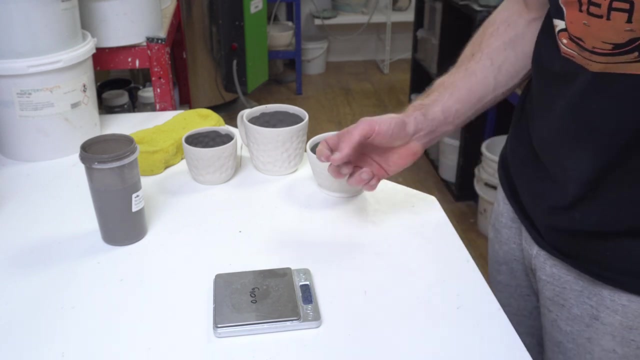 mug to get to this stage. this slows it down by a couple of seconds per application. it's a bit of a put it on there, fine, but it's worth it as far as I'm concerned for mugs. so I do it for anything that I'm putting floating blue on that's a mug and generally I'll do it for. 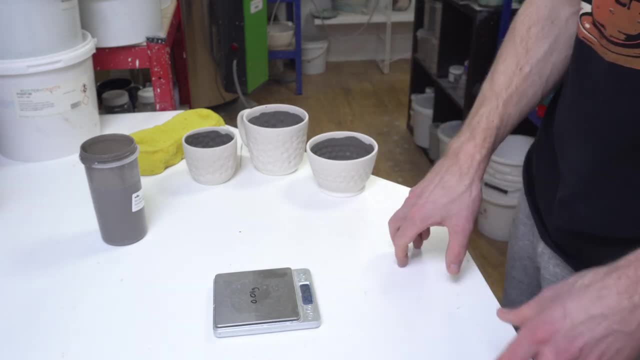 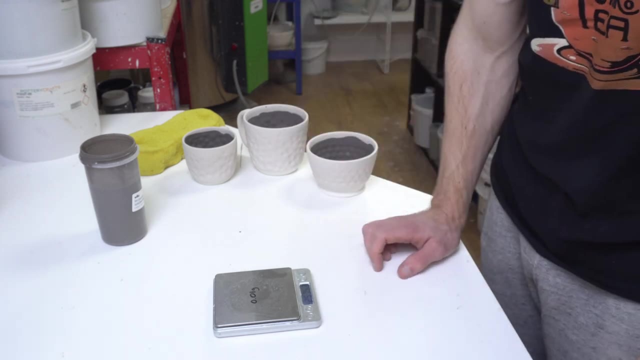 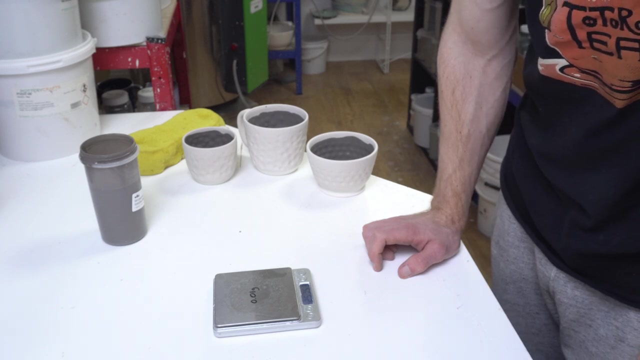 bowls. definitely, if you're going to do a set- which I am- of these um, you can be consistent across the entire set by doing this. again: glaze application- the same um, but really worthwhile. and then test tiles. test tiles are a huge one, because so many times I see test tiles on glazy where 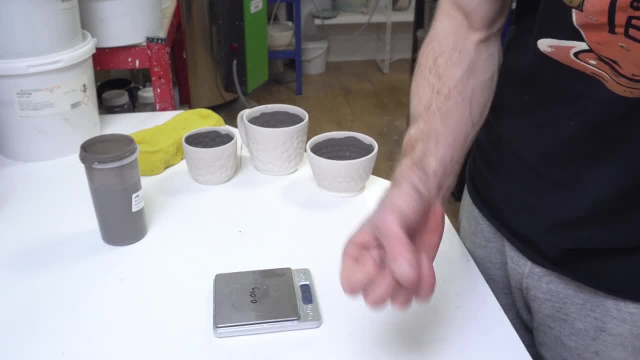 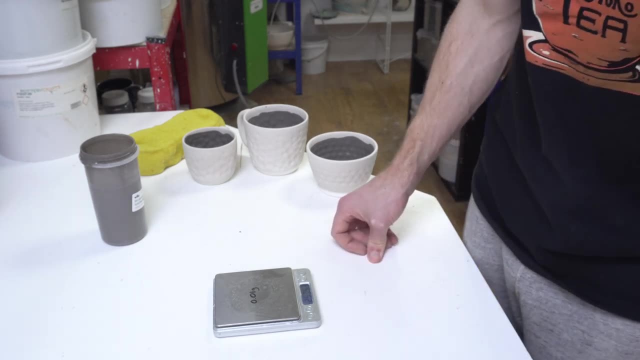 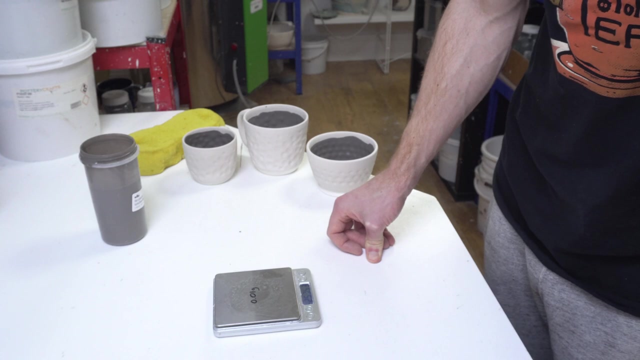 they don't look like the glaze that they're replicating. so someone will upload a test tile for a glaze. obviously I get notified when it's on mine, but I see it on other people's glazes as well and you can immediately see the application is way too thin and it can be because people's test tiles. 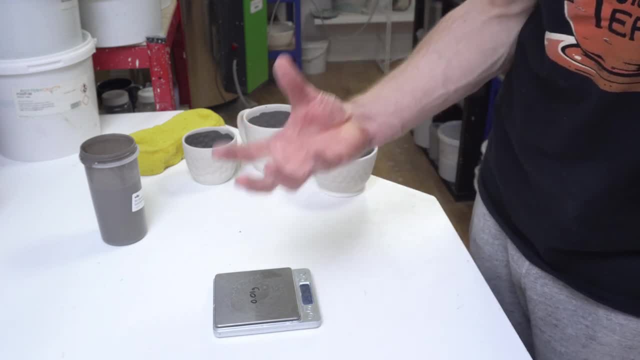 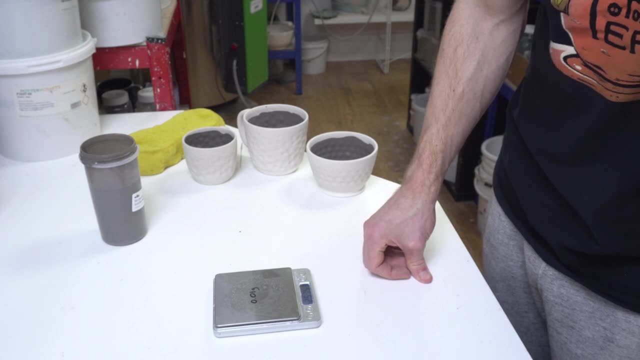 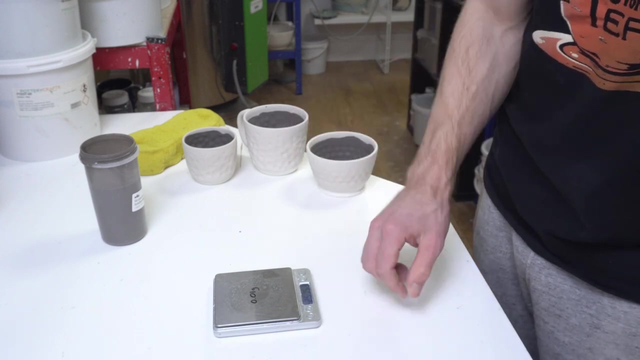 are quite thin so they don't take up the glaze the same way a thicker piece would, or it could just be that they're dipping in it. it could be that they've made a hundred gram mix and they've diluted it too much, but if you know how much of the dry glaze equivalent you're applying to, 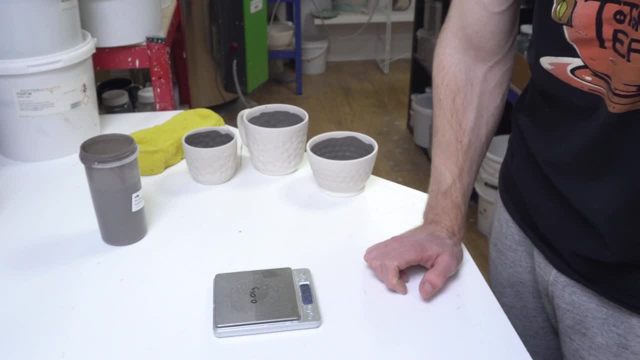 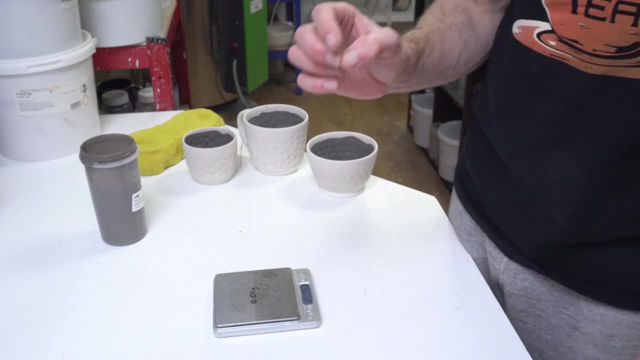 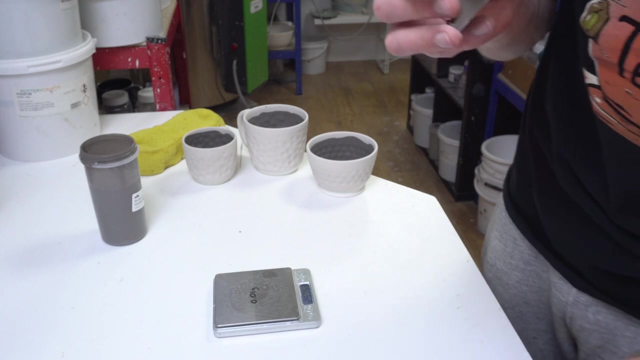 a test tile, then you have a really good idea um how that glaze should behave. um, and if in doubt, when you're doing test tiles, if the glaze isn't beading at the bottom. I don't have any particularly great examples because these aren't typically doing it, although you can sort of see. uh, let's see. 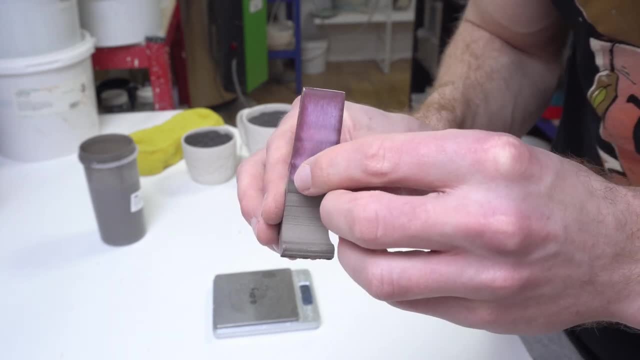 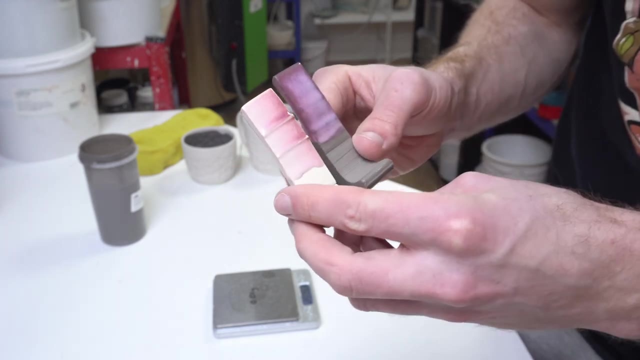 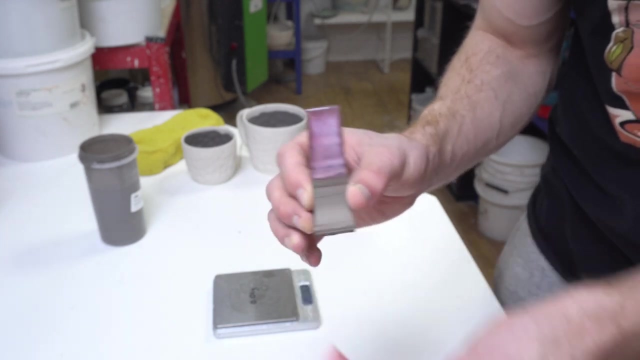 if I can get the focus on that, um, that bead at the edge. that's what you're looking for when the bottom of your test tile and I'll. I intend to post the recipe for this at some point. this is a glacier with two percent tin in it, so it's picking up the purple from that because it's. 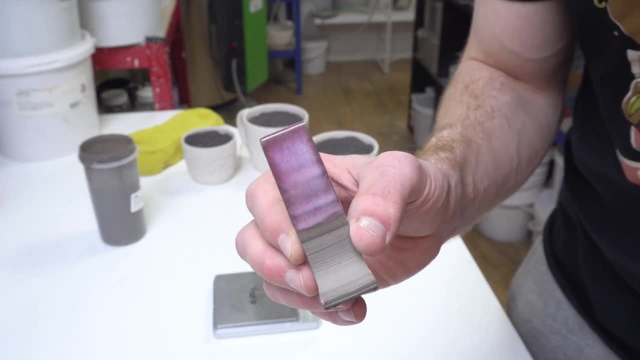 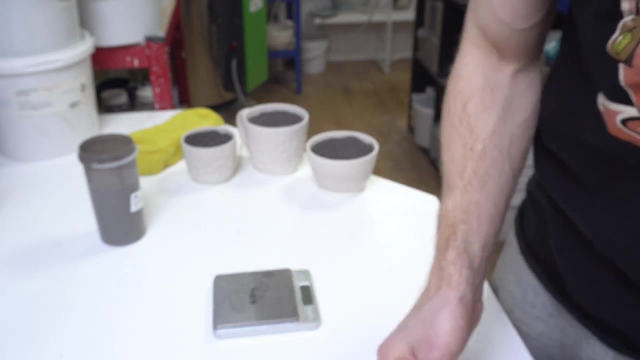 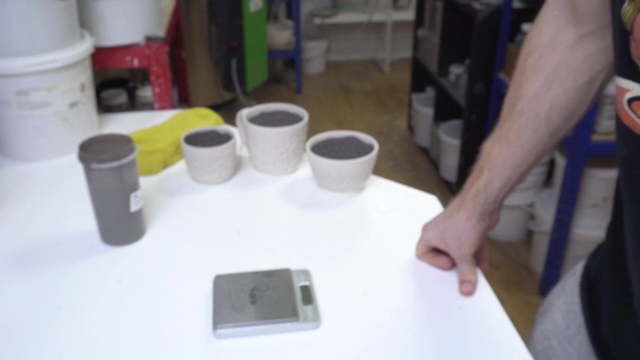 a chrome tin recipe focus. but yeah, you want that bead where it flows down if it's not getting thickness at the bottom. it's a thin application. once it starts to thicken at the base then you know you've put it on probably thick enough to get a good representation of what that glaze will do. um, but all of that can be. 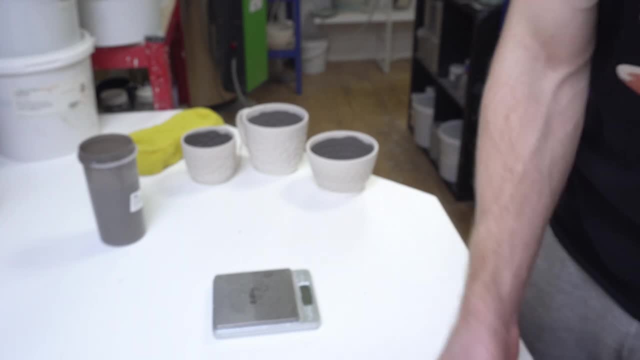 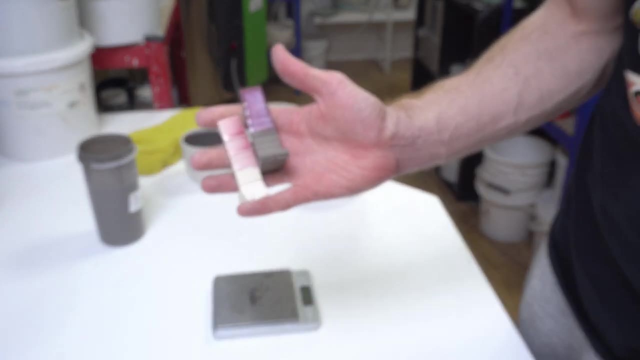 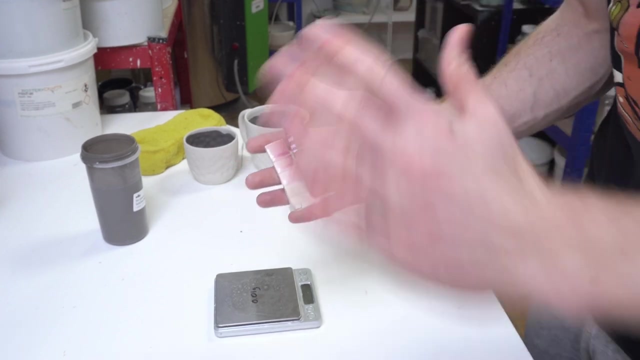 avoided by weighing your test tiles. and so if you've got test tiles like this, this sort of size, then I would ruin the focus. sorry I've not got this set on autofocus because then it jumps around too much. but um, the downside is that if I then fiddle, 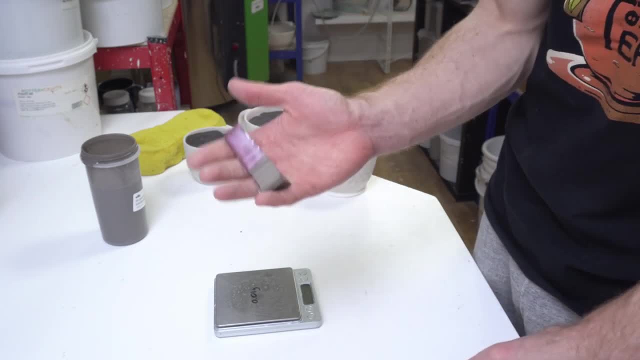 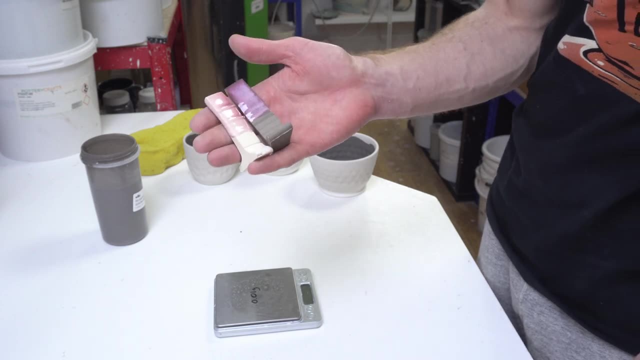 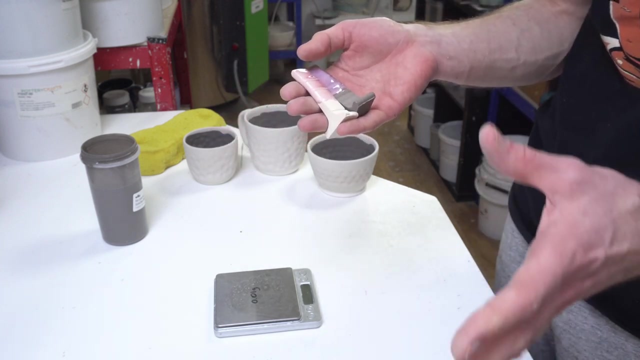 with it. it's completely wrong. yeah, if you've got test tiles this sort of size, um, I aim for upwards of three to four grams of glaze mix on them. weight increase. so that would be the equivalent of, say, two, one and a half to two grams of dry glaze mix on them. um. 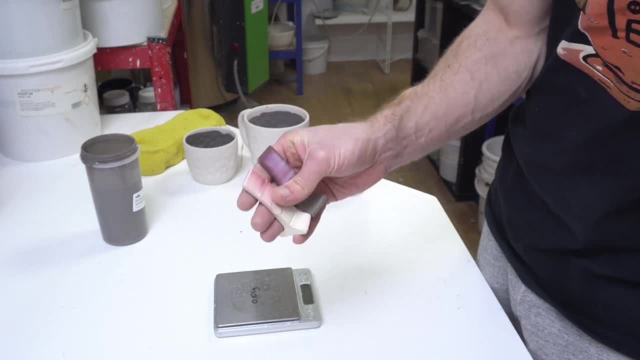 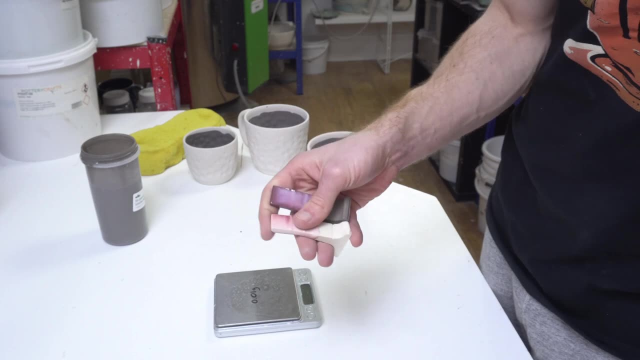 with that much glaze, you know that it's gonna be behaving the way you want. and by weighing them, you know, when you put them in the kiln, that you're not going to be disappointed with the application when they come out. you might be disappointed with the glaze, but you're not going to be sat there. 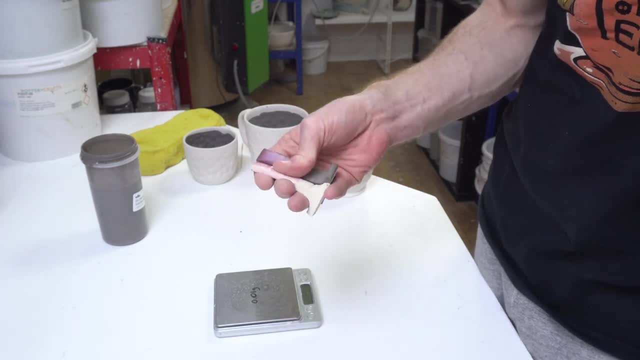 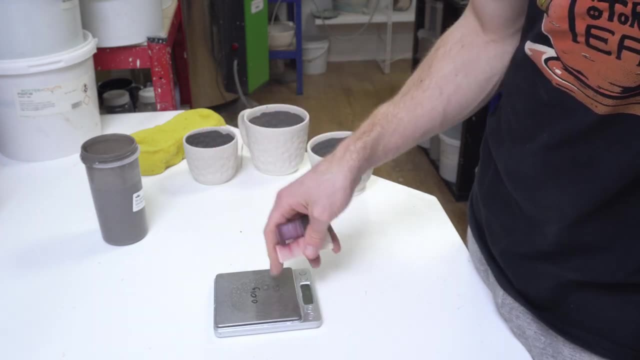 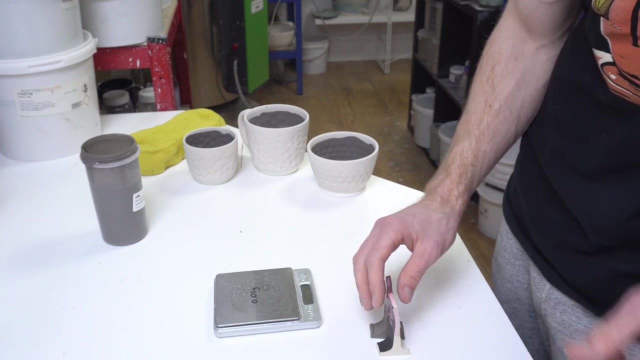 looking at the test tile going, I can't learn anything from this, because the application was off, so worth doing, in my opinion. uh, people should weigh their glazes more, because it's a great simple way to to vary as you go what the amount of glaze on a piece is and that at the end of the day, 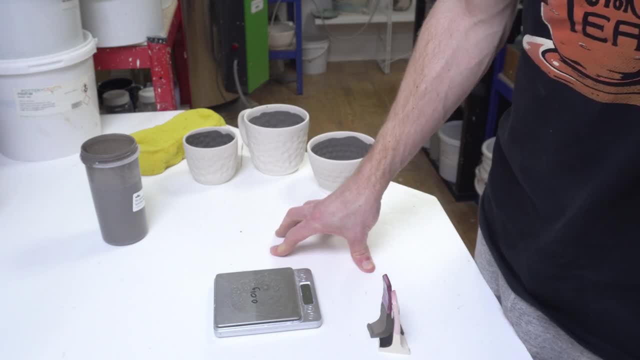 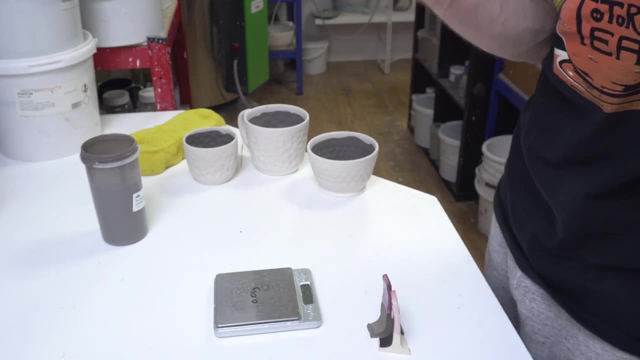 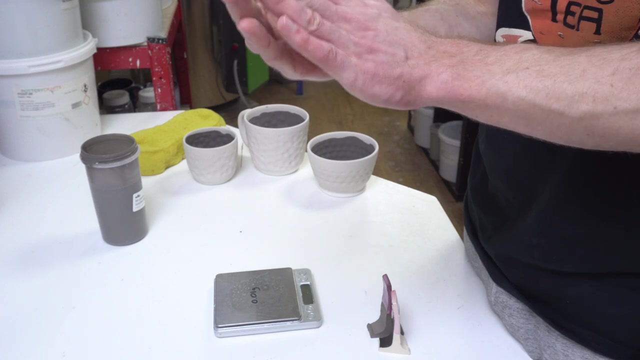 that's what you care about. it's not dip time, it's not even physical glaze thickness. I know some people have very precise measuring tools that poke a spike through a layer of glaze to the clay piece to see what the physical distance of glaze is in kind of microns. 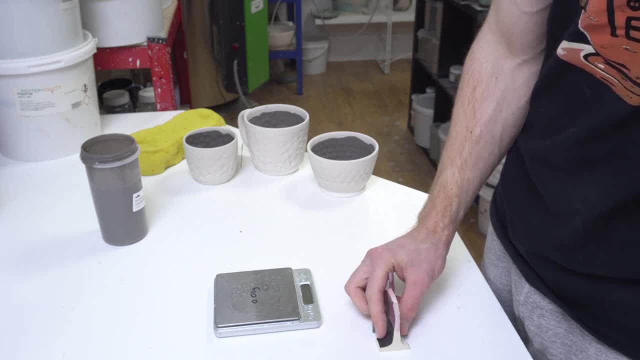 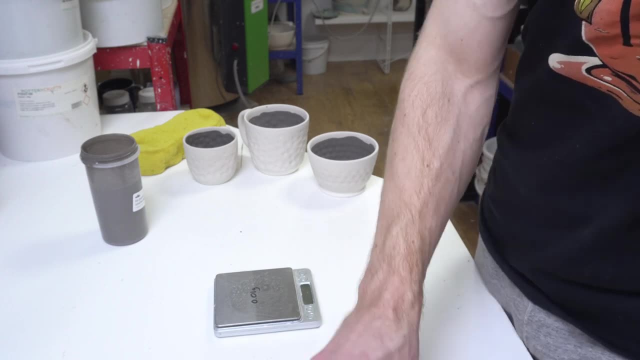 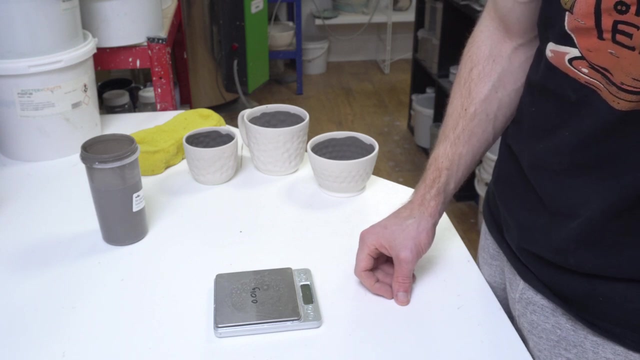 um, but back to how different ingredients will have different specific, different properties at different specific gravities. different ingredients will pack differently. um and so if you've ever used pretty sure mag carbs- the worst- but magnesium carbonate is so fluffy and um wood ash, if you've ever used kind of like um, I've got one of these.